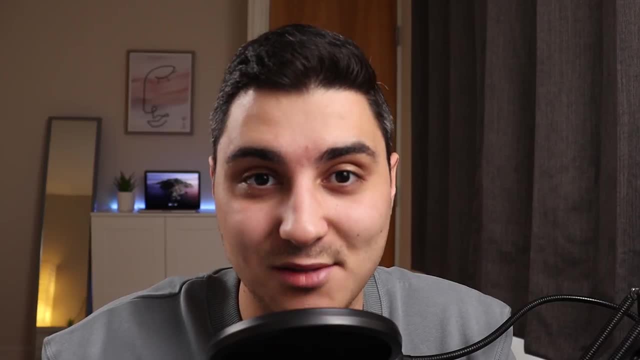 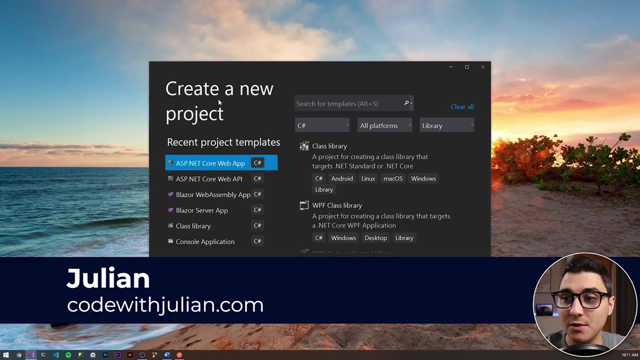 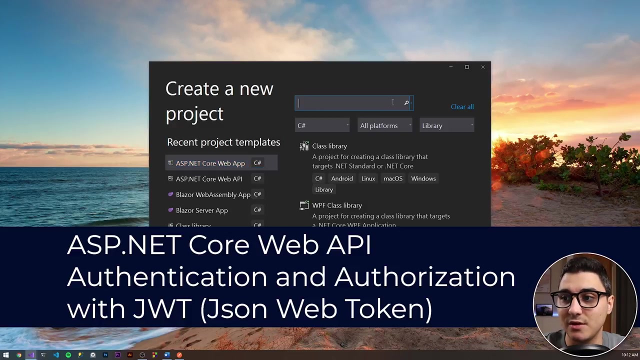 Today I'll show you how to add authentication and authorization in your ASPNET Core web application with JSON Web Token. So let's get coding. Okay, open up Visual Studio, create a new project. This will be an ASPNET Core web application. Select that. If you can't find it, search it in the 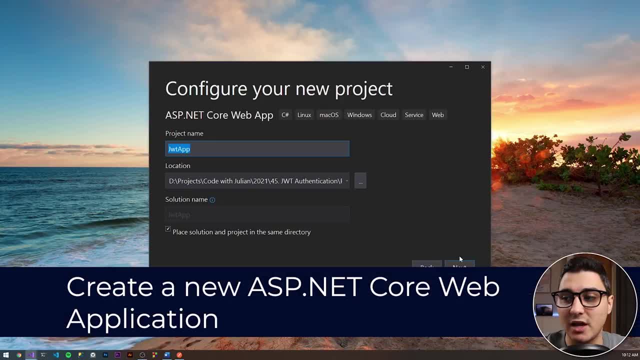 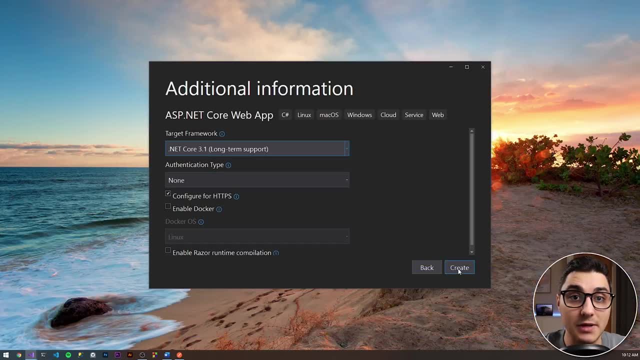 search bar right there, Click next, give it a name, give it a location and then click next again. And then here I'm going to choose NET Core 3.1, no authentication type and click create. So here we are. A few things that we need to do is to install three packages. So if you 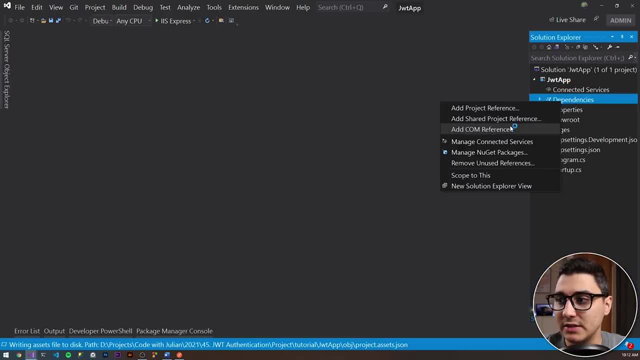 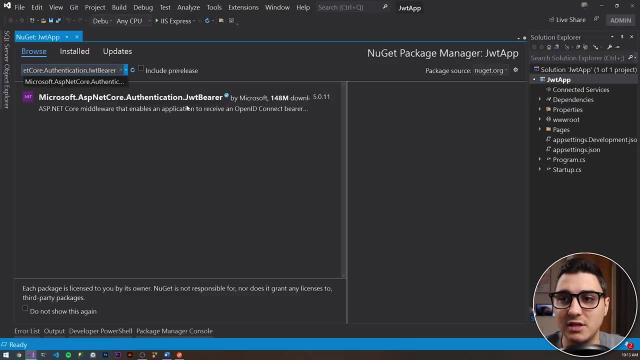 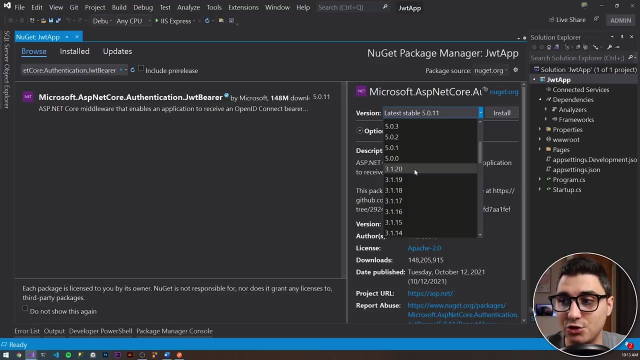 open up Solution Explorer, then right click on the dependencies and manage new get packages. The first one is Microsoft ASPNET Core authentication JWT bearer. One important thing to note is that if you have created a NET Core 3.1 application, then make sure you choose. 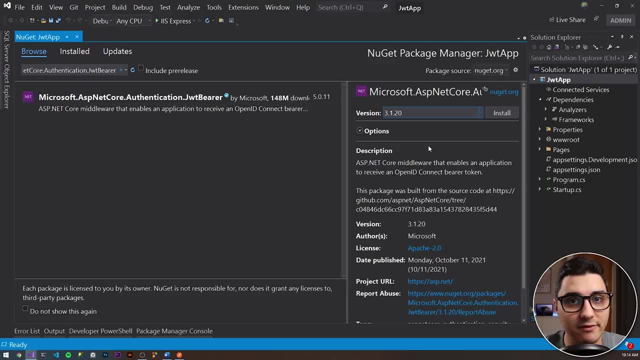 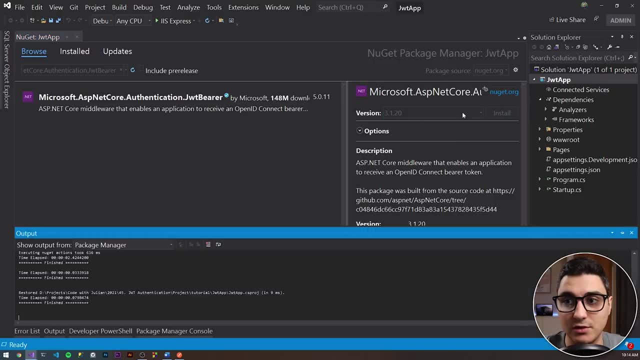 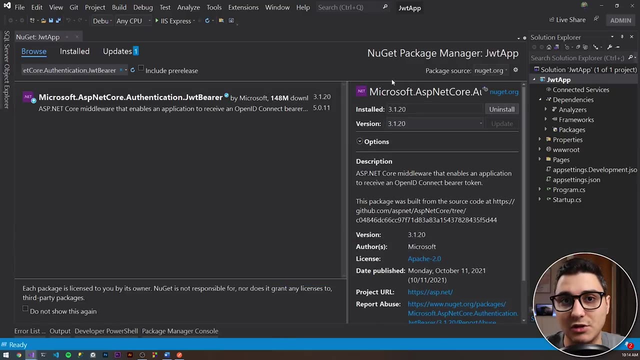 3.1.24 JWT bearer, because anything above that will not be compatible with the ASPNET Core, with NET Core 3.1. So just make sure that you choose that. If you're working with NET 5, then higher versions of the JWT bearer package will work, But in this case 3.1,. 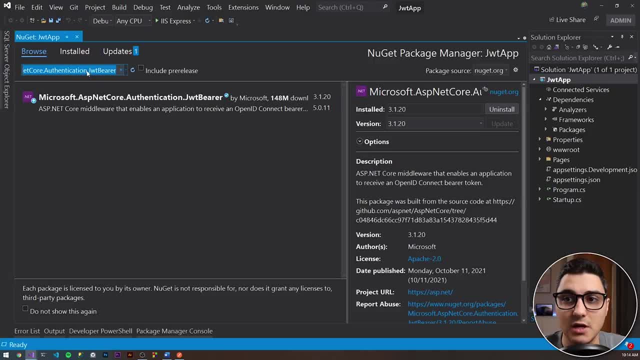 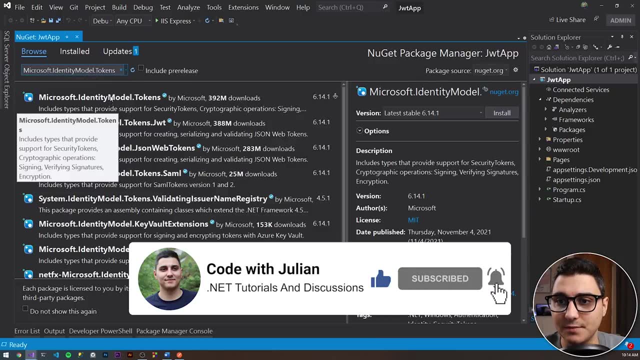 that's all you need to do. Okay, the next package that we need to install is tokens, so identity model tokens. This is it, And you can choose this one. It's fine for the rest of the packages to install the data stable versions. 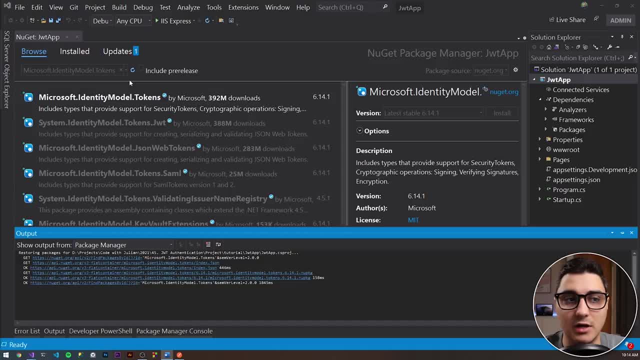 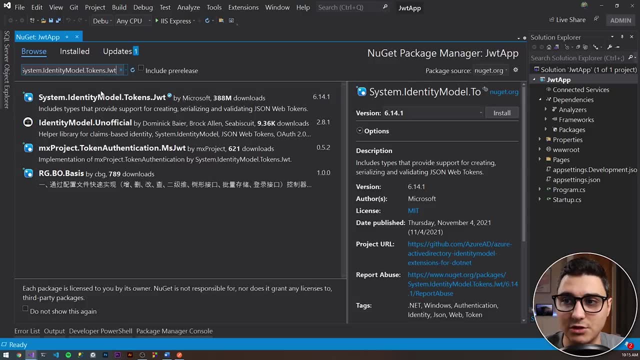 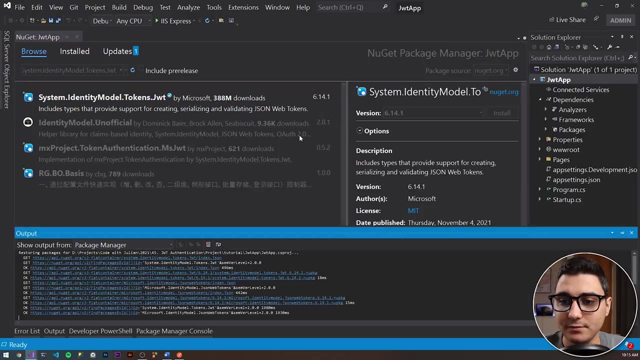 And then, last but not least, is identity models: tokensJWT. Okay, let's finish installing. So I'm going to paste in the description section all the all the packages so that you can go ahead and copy and paste them as you wish. Okay, so installing the latest one. that's finished. 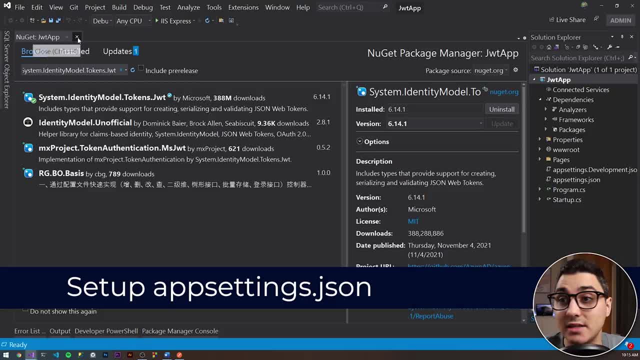 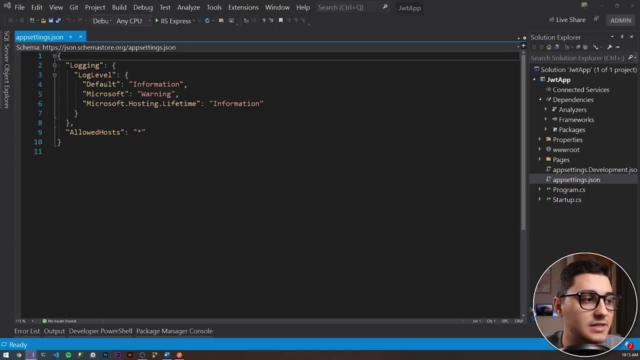 Okay, following the next step is to set up app settingsjson. So if we close everything and then we go to the root of our project and then open up app settings, app settingsjson. I've got a snippet that I've already created. I'm just going to paste that in. 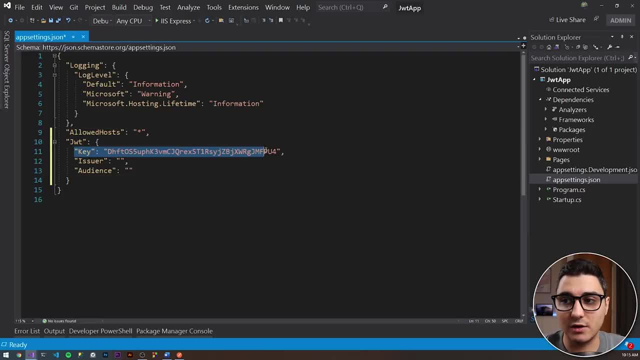 So this is a new section JWT that I have created that's got a key that's randomly generated, link in the description with a website that's just generated a random string of characters and numbers, And then we've got an issuer and an audience And we need two addresses here. 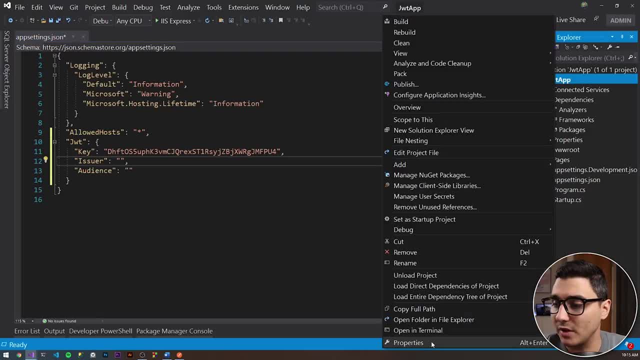 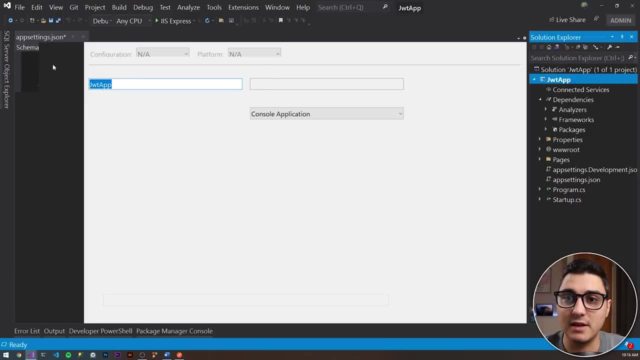 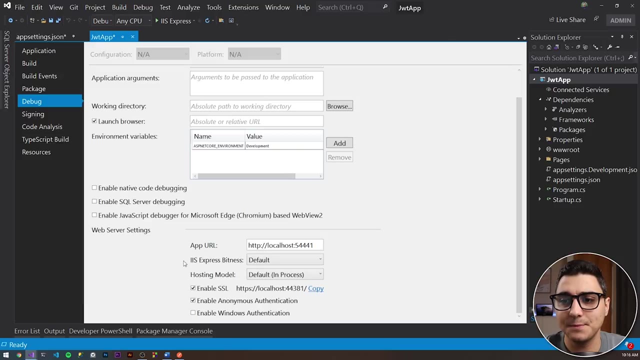 which in our case are going to be similar. So if we right click on the web project, on the web app, and then go to properties and then navigate to the debug tab, scroll down and you will see that right next to it. So in the web server setting settings section we've got enable SSL and then we've got an. 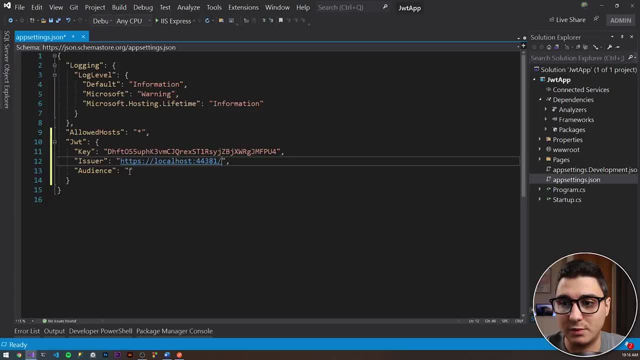 address here. that URL is what we need to paste in here. So both the issuer and the audience, or the server that's going to issue the debugjsonjson- that's the unique thing about that issue- the JWT token and the audience- the one that's that's gonna use it- are gonna have the 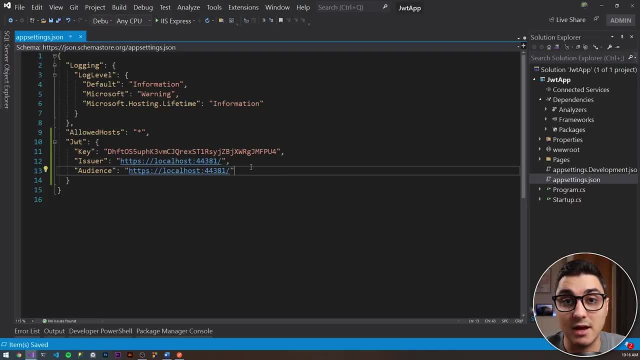 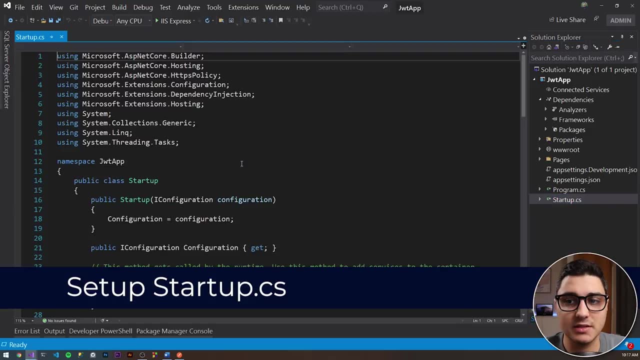 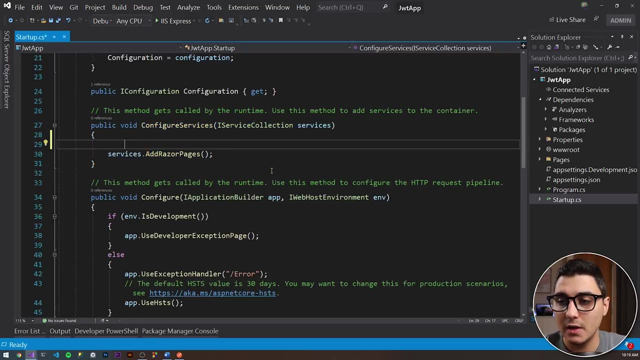 same address. so that's it with setting up app settingsjson. following, we need to set up startupcs file. so if we open up startupcs and scroll down to configure services, so we've got that method right here, it should be on line 24, okay, so inside the configure services, inside startupcs, we need 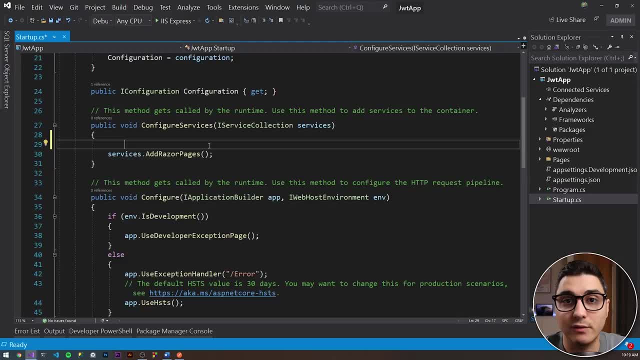 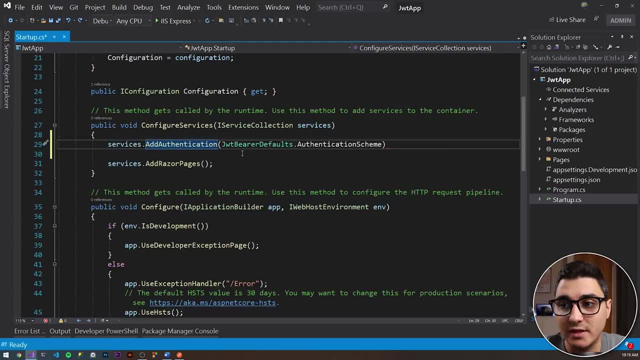 to add the configuration part for the JWT bearer. so that's the first thing. so we do servicesadd authentication and then in here we define JWT. we say we pass in the authentication scheme as JWT bearer defaults and that's not it. by the way, if you haven't got this already imported in your 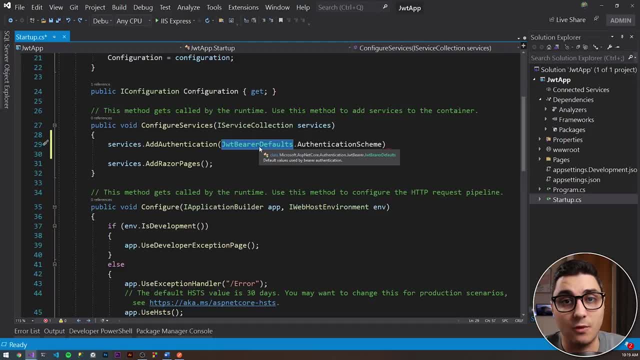 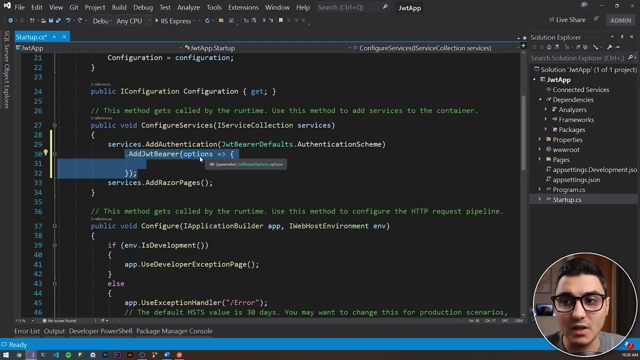 startupcs, just press control dot and then hit enter and then one of the packages should just import automatically inside the inside, inside startupcs. then following, we don't put a semicolon at the end, we do a dot, add JWT bearer, and then we define an options object that we need to define. so we need in order to in. 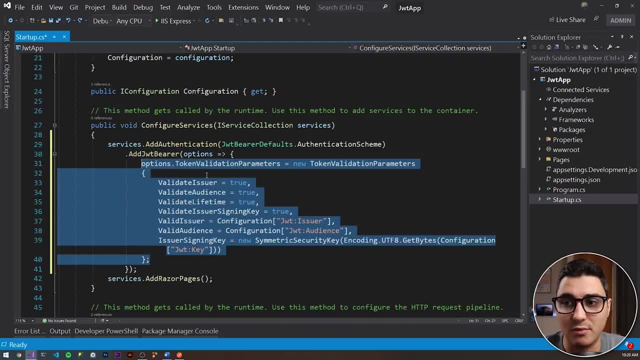 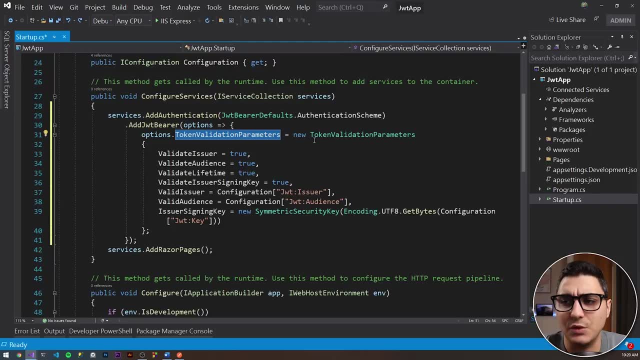 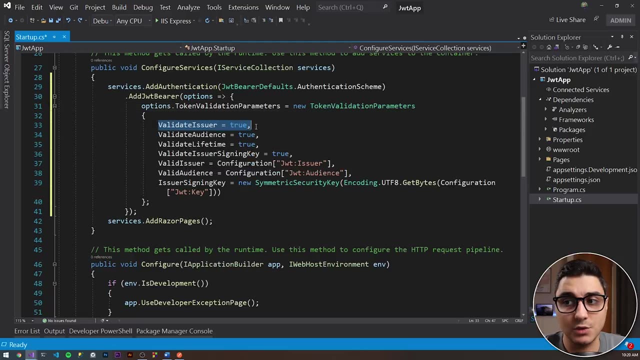 order for this to work properly, we need to set this up with our custom properties. we've got our custom options. we need to define the options- dot token validation parameters- and obviously we need to initialize that with a token validation parameters object. so we need to tell the API that every time you receive a request with where you've got the authorized tag in it, then validate the issuer that we have defined earlier inside app settings- dot json, obviously validate the audience as well, validate lifetime and then validate the issuer signing key. so we need to validate that as well if we are going to provide a signing key. 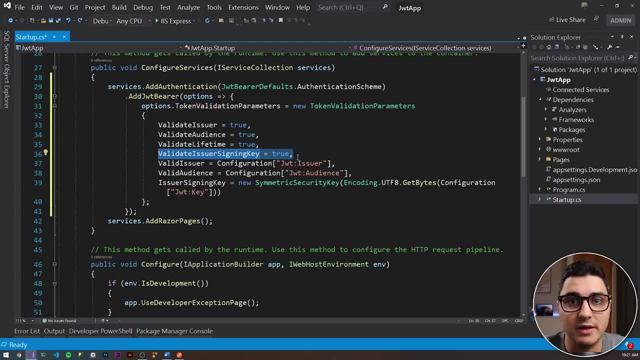 it could be optional, but just to make it more secure, to add an extra layer of security, we are going to define a private key. then the valid issuer that we define is from the configuration, so from app settingsjson, and we're accessing it using jwt colon issuer. 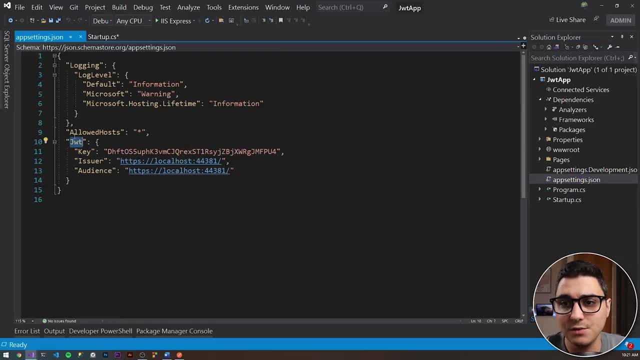 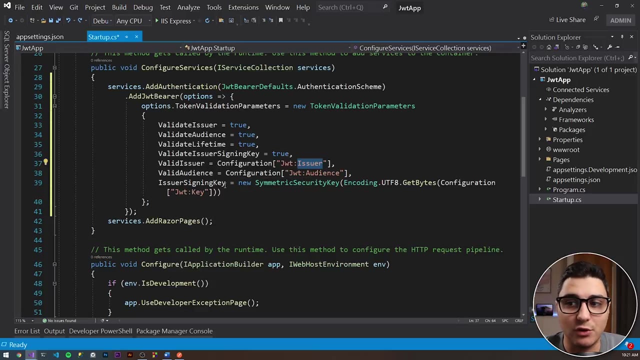 that's the path to it, right? so jwt is the section and then issuer is the actual value. so this is what we're going to import in there and this. this is better than just pasting this string in here, because this is an app secret. so when you get to deploy this, you'll obviously be able to replace. 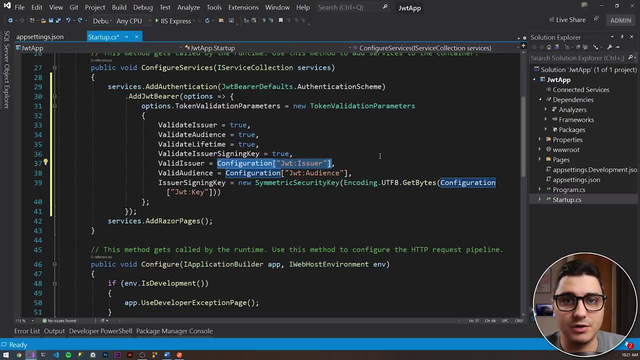 the, the value in app settingsjson, with the issuer on the server and the audience address on the server and so on, so that, following we define the valid audience that this is going to be, that the token will be validated against in here as well, and then the issuer. 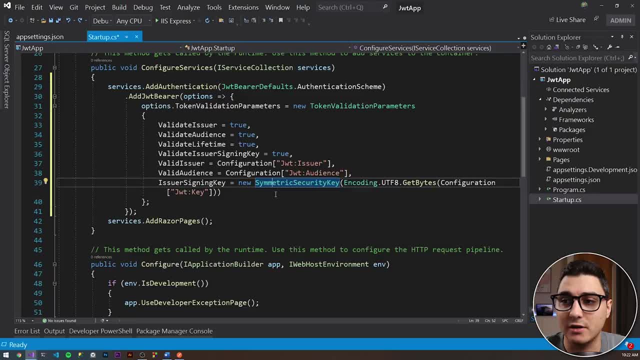 signing key. we are doing a symmetric key, so we're creating a symmetric security key and obviously we're encoding that jwt key so that we can create the symmetric security key. so that's how we, that's how we define the options of the token validation parameters following we need: 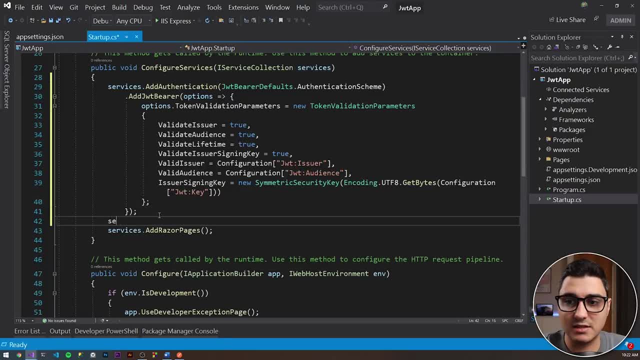 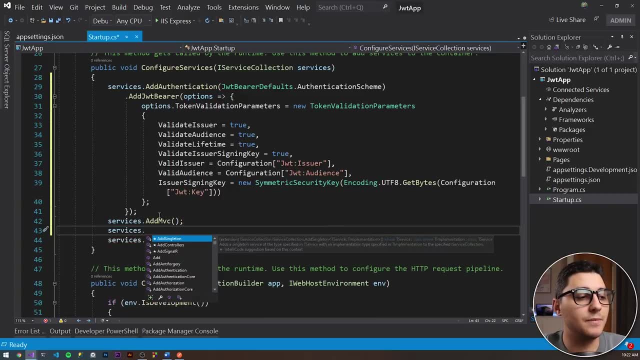 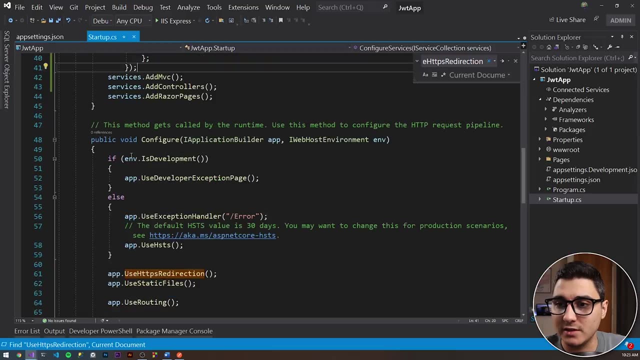 to add a couple of lines again in this configure services method. that's going to be: services dot add mvc and services dot add controllers, and that is it with configure services. then in the next part, what we need to do is add a couple of lines, a couple of configurations inside the startupcs configure. 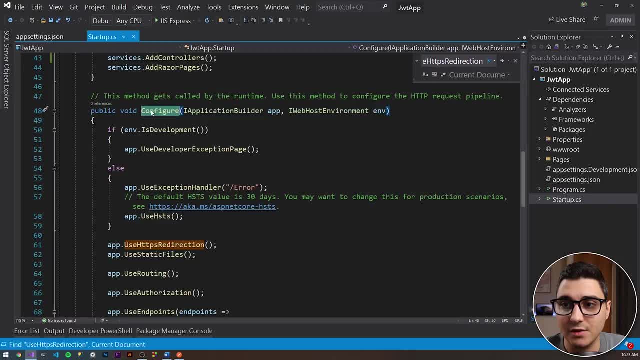 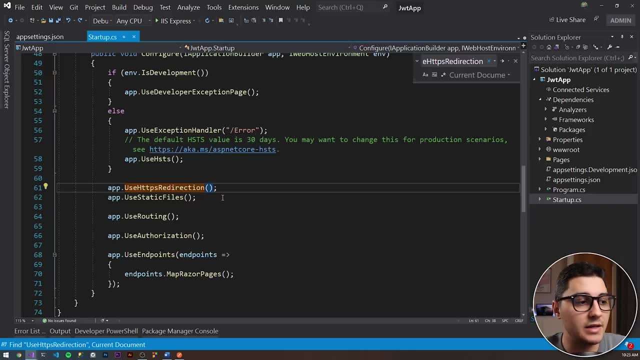 method. so this is different to configure services. in here we we are aiming for a configure method and in here we need to add authentication and map the controllers, because if we don't do that, when we get to create the api controllers that we're going to use throughout the application. 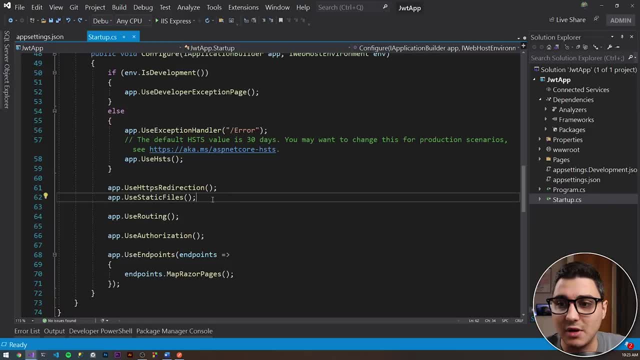 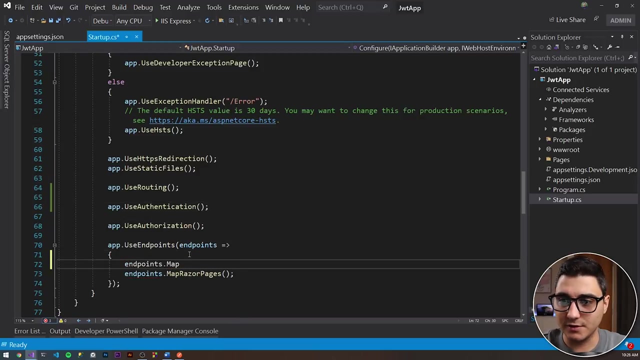 we won't be able to access them, so very important to do this step. so the first thing that we want to do in here is app dot use authentication. yeah, so that we can, we can allow for the api endpoints to authenticate the users. and then, last but not least, endpoints, dot map controllers. 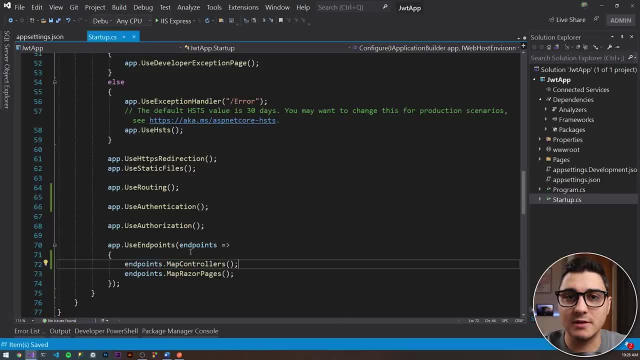 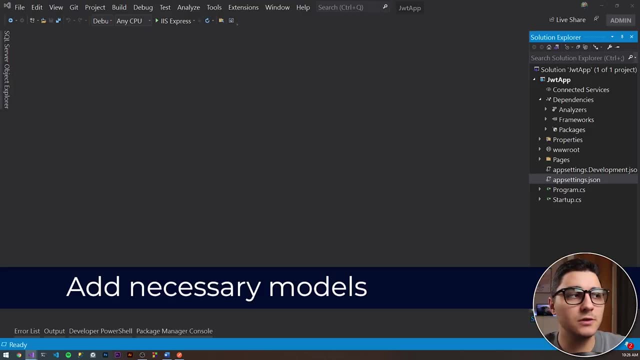 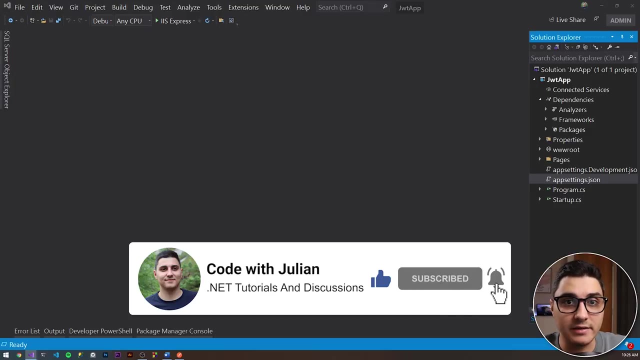 map controllers. that's it with setting up startupcs right now. let's add a models folder to hold our three models. one will be the user model. uh, that's going to hold all the data about a user. so this is going to be some sort of like an asp net user entity in the ef core, but obviously 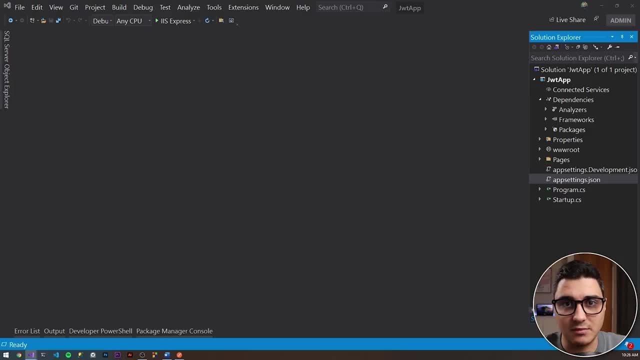 we're not going to work with an ef core database, with the sql server database, uh, therefore, we're just going to simulate the presence, the presence of it. uh, so, user model: user login: that's going to have only username and password and the user constants, that's going to be some sort of like. 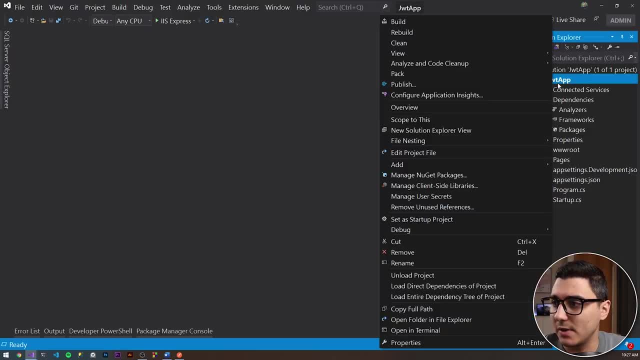 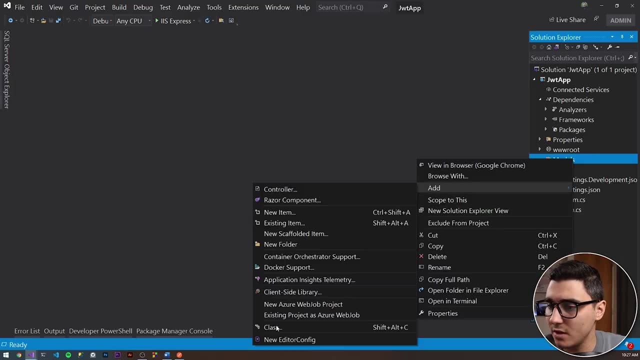 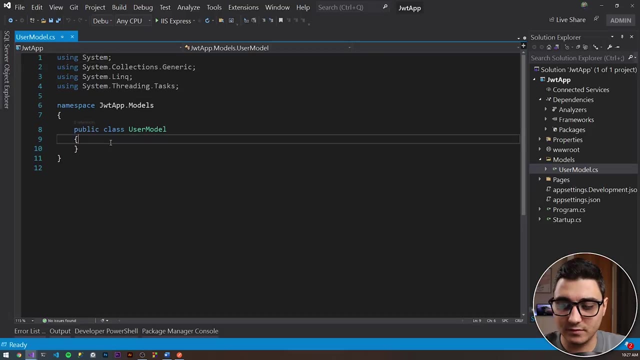 a database holder for us, okay, so, um, let's right click on the project, add a new folder, models, and then in here, like i said, three classes. the first one, user model. user model. this is going to be a public class and i'm pasting in the the properties right now. 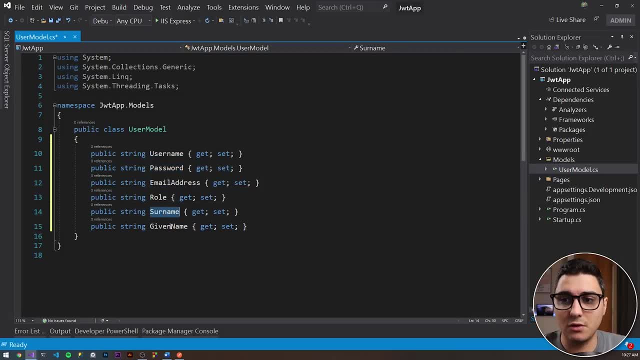 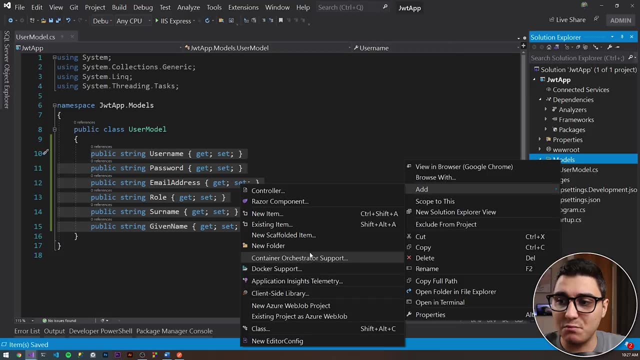 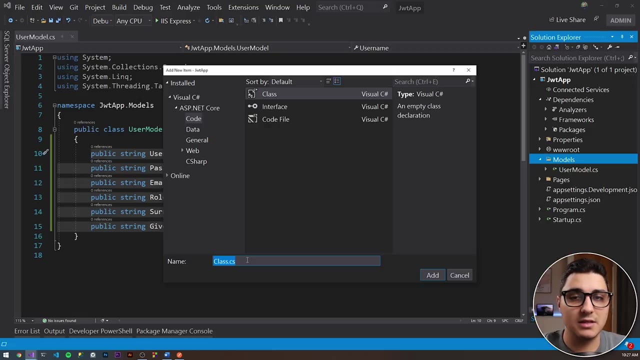 so we've got username, a password, an email address, security role, a surname and a given name. so pretty simple. then the second one will be user login and obviously you can pass in the API the username and the password, but it's it's better to do it like this. it's best practice, you'll see. 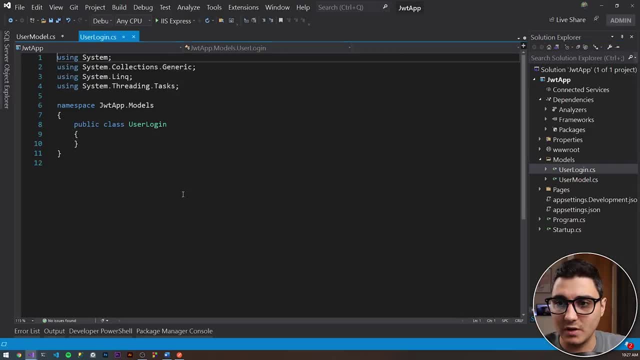 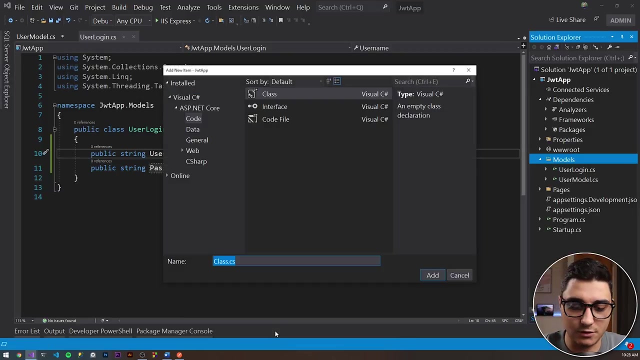 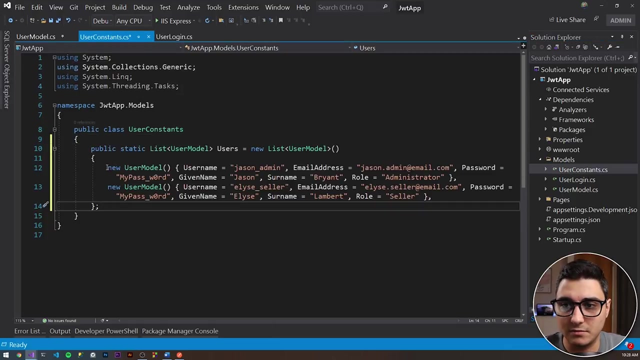 what I mean. so user login, and this is gonna have just a couple of strings: username and password, that's it. and then, lastly, the user constants. so right-click, add new class and let's call this user constants, and this just holds a list of two users that I have already created for us. one is called Jason admin. 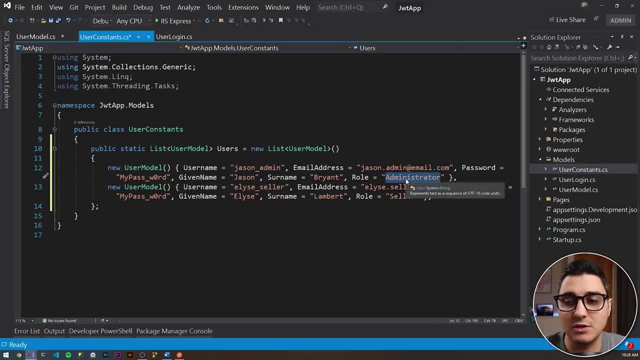 and it's an administrator. it's got a roll of at you but administrator, and then one is called the other one is called a list seller and it's got a security role of seller. so this is it, with this step, with setting up our models, that we're going to use. 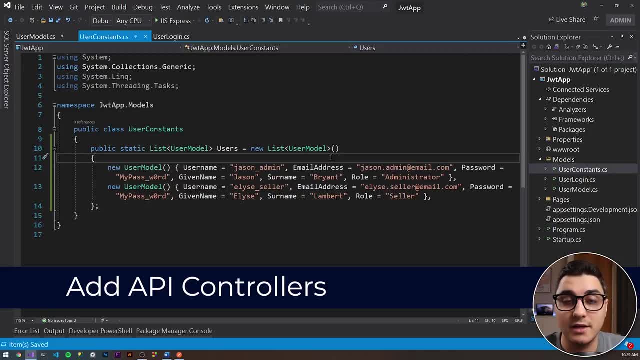 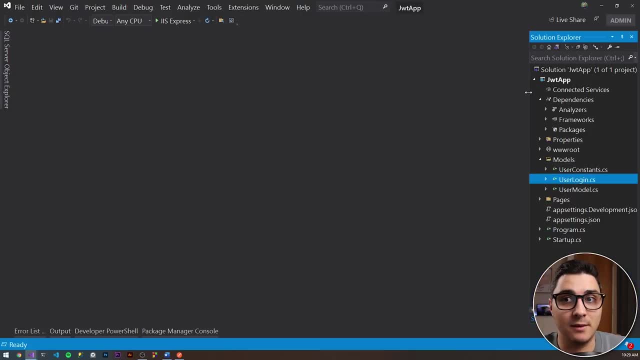 throughout this application. okay, following here is the meaty part: we'll add the api controller. so the first api controller that we want to add is the login controller, which is the one that will authenticate the user as well as will generate the token for for the user, based on the user. 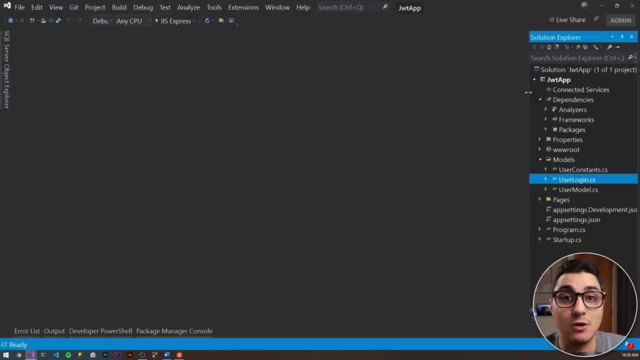 details that are found in the database, based on the user name and password. so let us create a controllers folder, so controllers. then in here let's create a, an api controller, so right click, add new item and then type in api, if you don't already see it. and let's call this login controller. 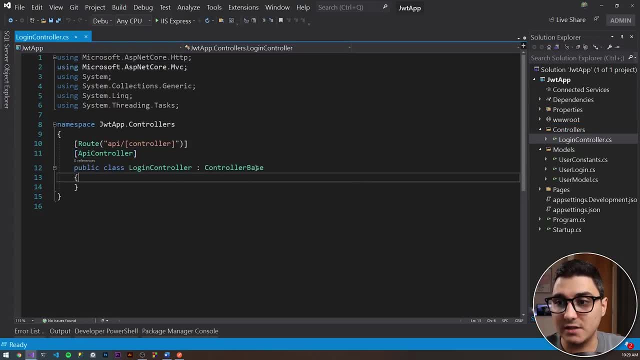 so this is an api controller that's inheriting from controller base. okay, the first thing that we want to do, obviously, is to initialize the, to inject the i configuration so that we can have access to all the details from app settingsjson. so i'm just going to find 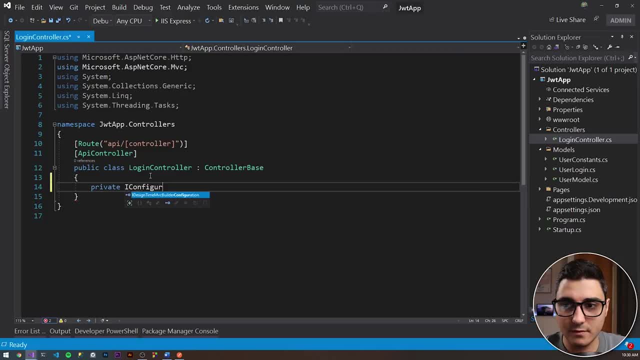 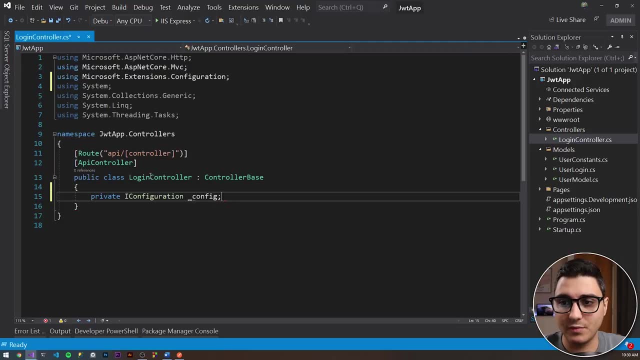 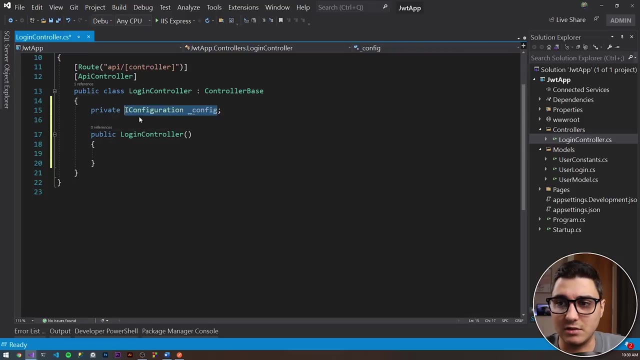 a private i configuration property at the top of the field, at the top of this class. that's going to be called config, and then if you type in ctor and double tap, then we can actually inject this. so i'm just going to copy and paste this here without. 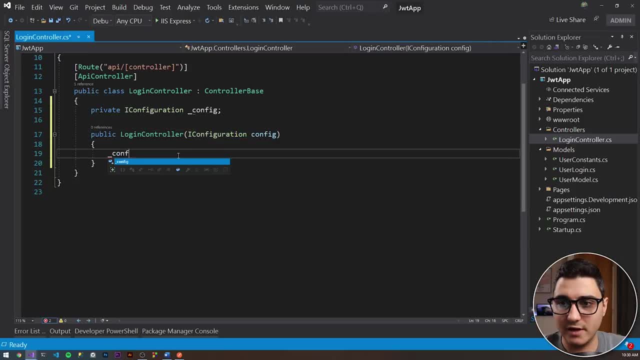 the underscore so that i can do config. dot config equals to the config object that's passed in, so this is how we inject things. then the very first method is obviously login, so this is going to allow anonymous. this is an annotation that will prevent the authorization process. the 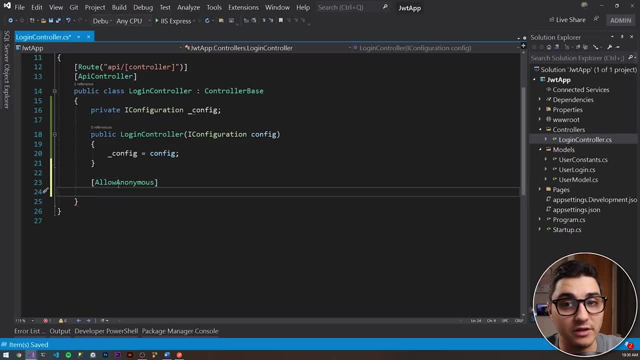 authentication process to happen at the point of the authentication process. so i'm just going to call this method, because this is the very first thing that the user is ever going to call in this application. the login method, obviously, if they're not already logged in. okay, so this is a http post. 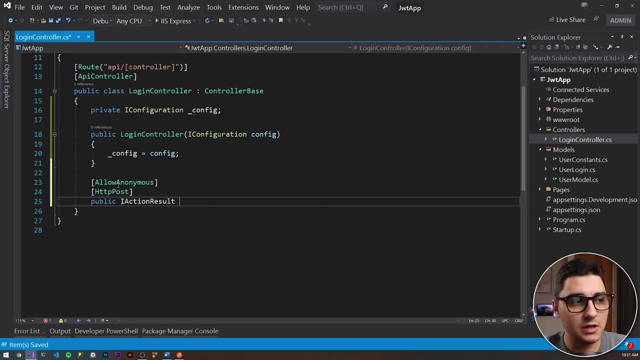 and then this is a public returns, an i action result, and it's called log login. okay, and this is going to take from body, oops, so from body- a user login object and let's import that really quick. let's call this user login. so, again, this user login only has username and password. we could have easily just 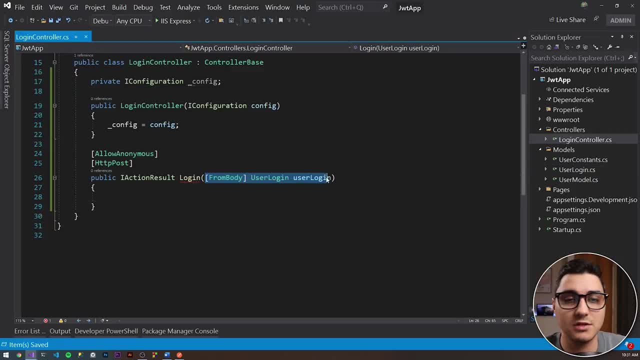 passed in those two strings in the, in this, in the parameter section. however, it's best practice to just wrap it in a in a dto, in a data transfer object. so in here, obviously we're not going to have all these methods yet, but we're going to create them. but the very first thing to do is to 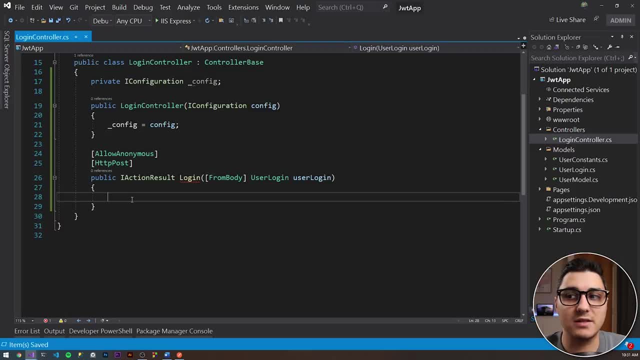 do is to grab the all the user details based on the username and password. so we do var user and then we call a method called authenticate. but wait, there is no authenticate method. we're going to create that in a bit. so let's pass in user login and then, if user is not null, 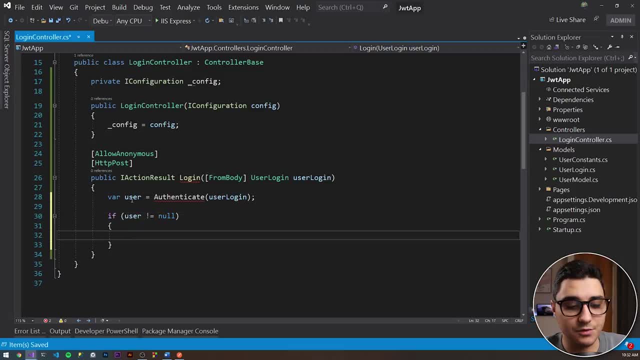 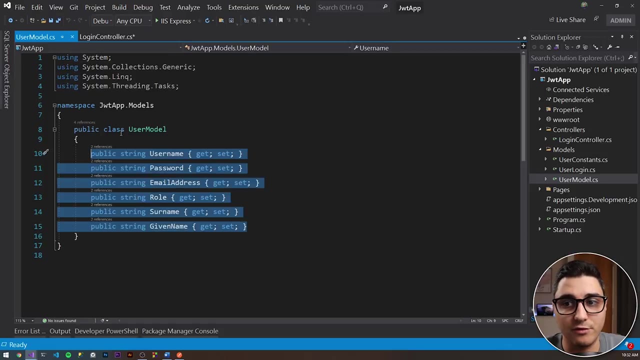 yeah, uh, then let's generate the token, so var token equal to generate, and then we pass in the user. uh, this user will contain all the user details. uh, this is going to be uh, created from um user from from the user model class. okay, uh, and then obviously we found it here, so let's just 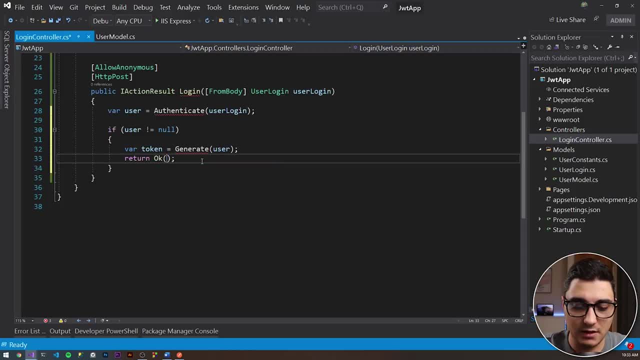 return this token in an okay object, um, in an okay response. yeah, but then if we uh couldn't, uh, if we could not find the user, then let's return not found, not not found, with a message user not found. so that way we know that the user name or user password are wrong. 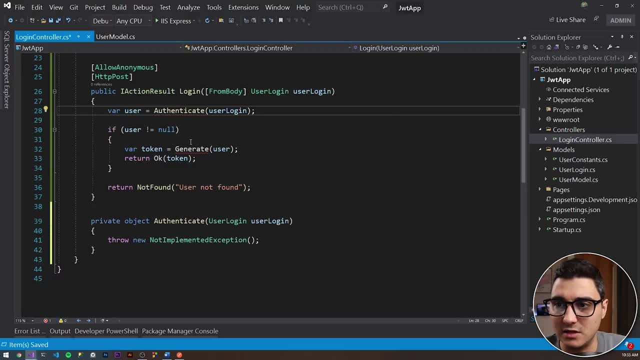 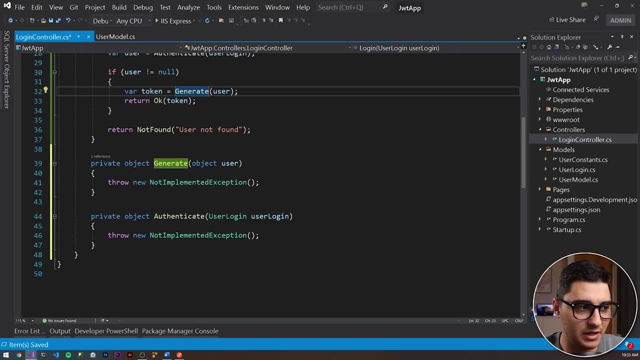 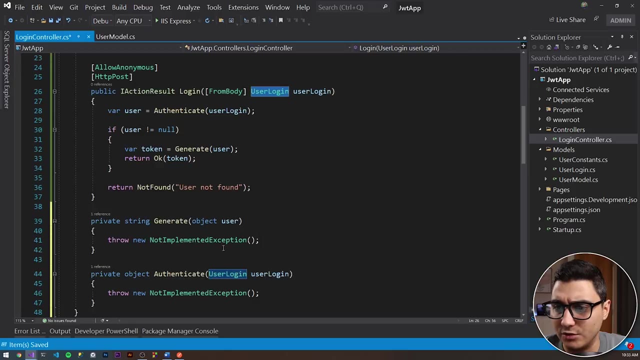 okay, then let's generate these two methods, and this is the authenticate and generate, and to do that, you just uh, control, dot on them and obviously the return types are a bit messed up, because this generate should just return a string and should take in a user model, user model and then. 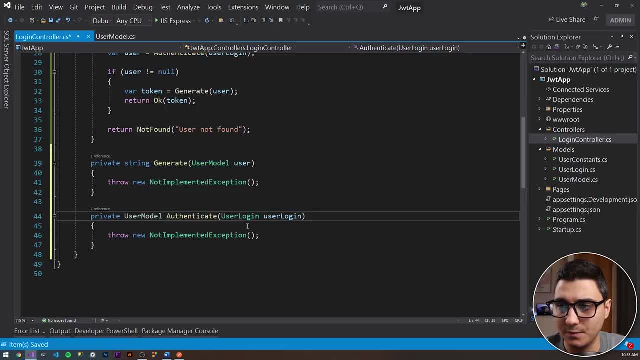 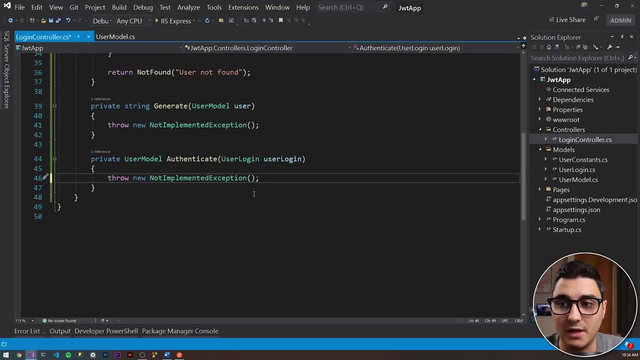 this authenticate should return a user model and, uh, yeah, it takes in the user login. so we're good to go now. so let's first work on the authenticate method. so the first thing that we do is, obviously we return the current user based on the user login information, so that, um, when the user name 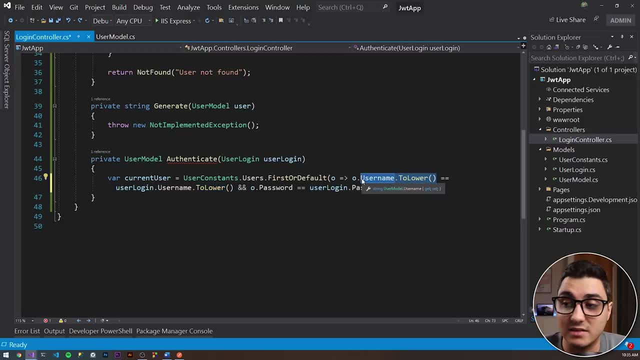 obviously i'm doing to lower because the username is case insensitive. it's like the email address in the login form, um. so if we found the username that's matching the uh login username, um that we have provided as part of this object that we're passing in, but then if the password 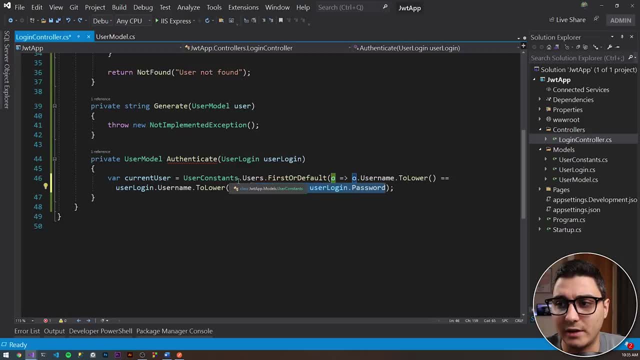 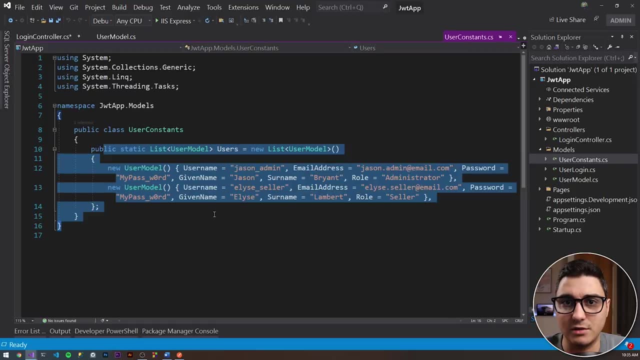 is the same as the password. then return the, return the entire uh object from the user constants, uh dot users. so this will be uh this class right here. you could have just easily uh call it a ef core to do this for you. um, so use ef core with sql server database. but this is not the point of 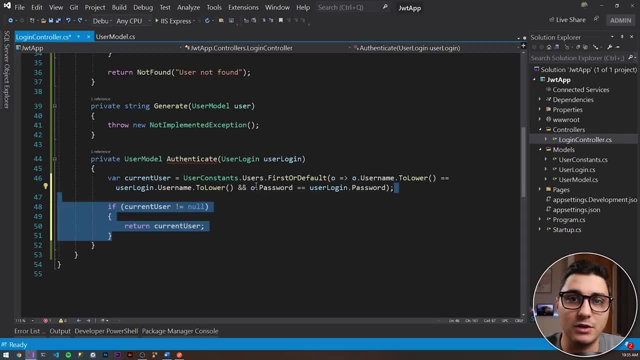 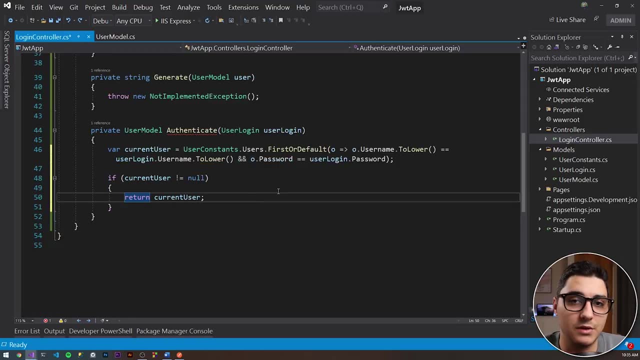 this tutorial. okay, so once we have that user, obviously we don't know whether or not it's going to be found or not, so we check in. if the current user is not null, then just return the current user with all the details that you found about it. otherwise, just return null. 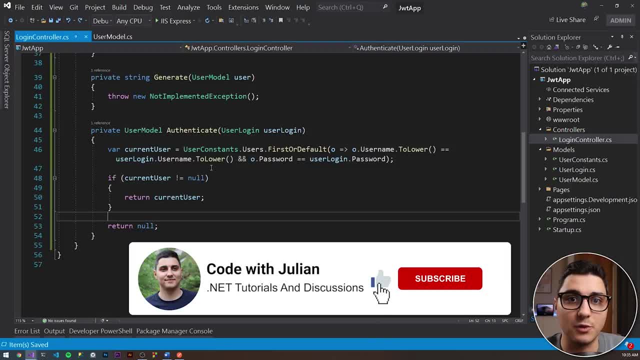 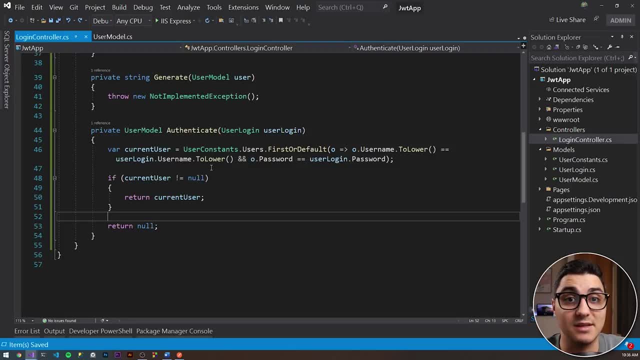 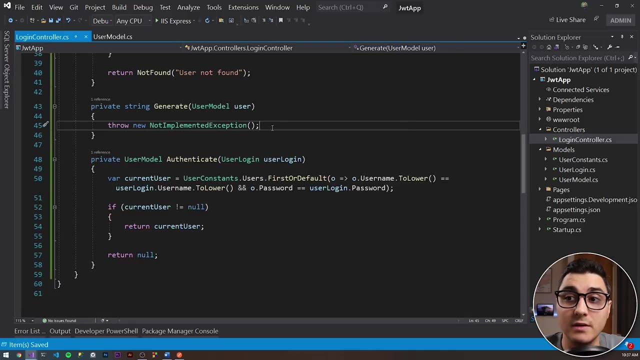 so that's the authenticate method. worth noting that this is not a proper authentication, so you shouldn't do this in your application, in your production application. this is just for testing purposes, to simulate the process of authenticating the user and basically validating username and password. okay, next thing is to configure the um generate method. that's gonna, this is gonna. 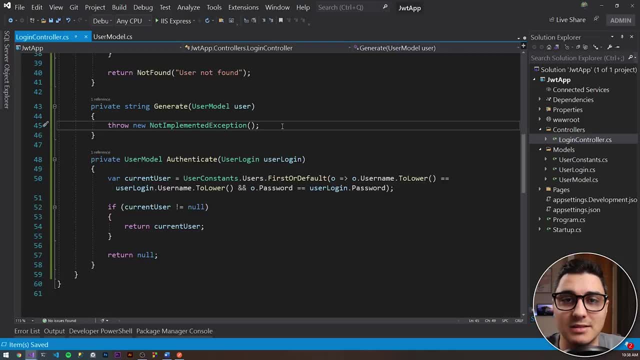 generate the jwt token based on the user details that we grabbed from our so-called database. the first thing to do is to grab the security key and define it as a symmetric security key, and this is, if you remember, the same exact thing that we have done inside the startup. 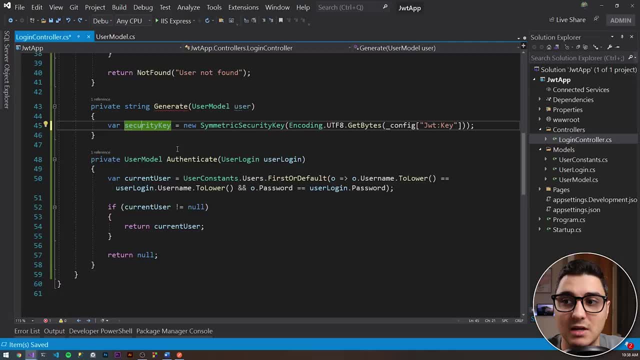 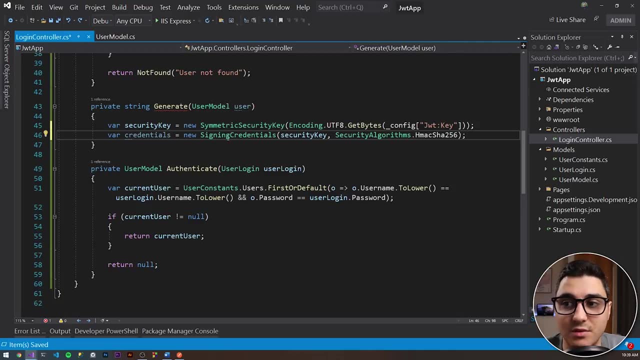 class. we're grabbing a randomly generated string of characters that's gonna be um, our public string. uh, then the second thing is to define a credentials object based on the security key. so the signing credentials that's gonna be um in included inside the jwt token, the job token. so here we're using. 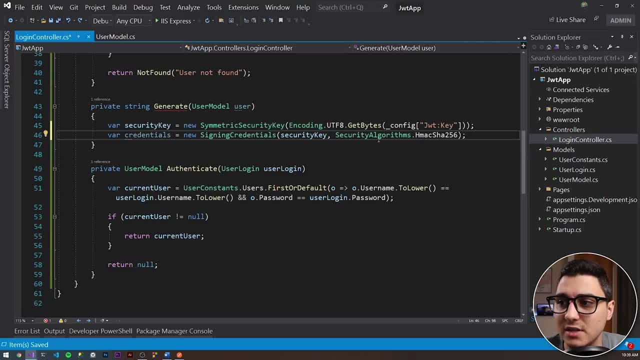 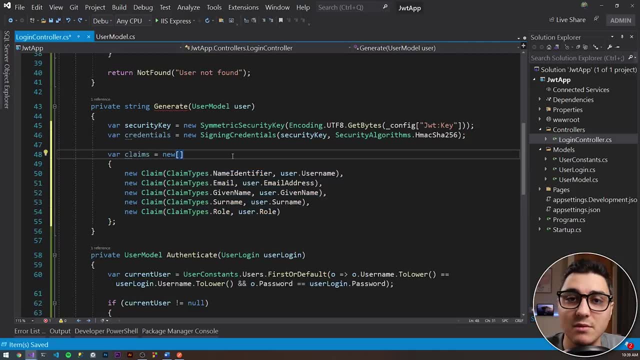 sha256, uh, hmac, sha256, obviously as a, as a security algorithm, as a hashing algorithm, and then we have the criminality of the defense mode, and it's a very kind of basic method that we're using to uh uh uh, simulate the, uh, the health of the user, and but a couple of things that i wanna point out. 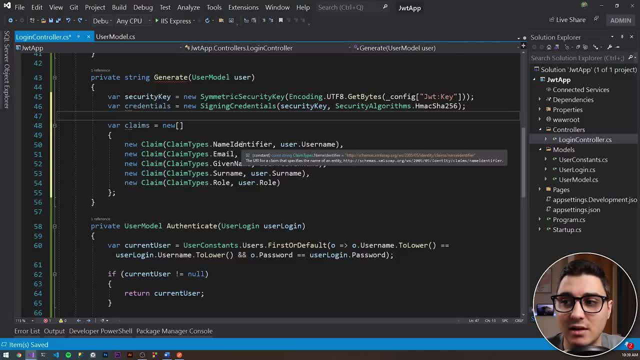 uh, we also have a feature called the ua claim type, which is that a lot of people know about the claim type. that is basically a bunch of form Emperor claims and they're basically a bunch of claims and claims are just a way to store uh data about the user or about the um, the, the, the process. 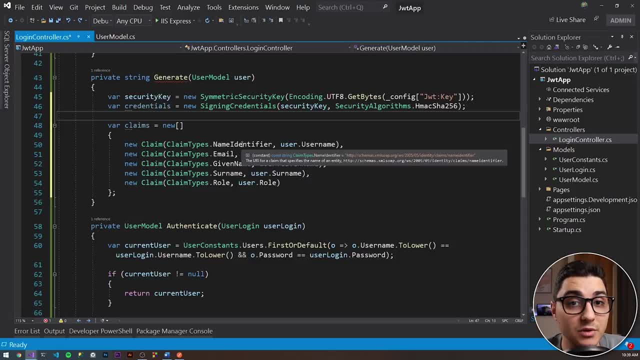 uh, and what we're storing at the moment is a bunch of claim types, and these are um already registered, the different types of claims and the components of a JWT token. so if you haven't already seen that, check out the description after this video or check out the end cards and you'll be able to see it. okay, so we have a name identifier. 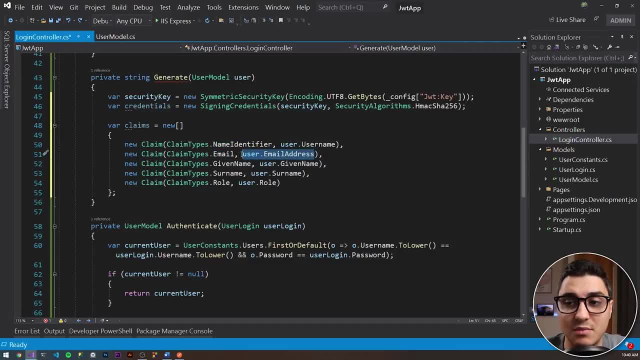 an email address, that we're just grabbing the user's email address and then a given name, surname and the security role. and the security role is important because we can actually use that to provide some level of access inside our api's. okay, so, after we define our array of claims, the next. 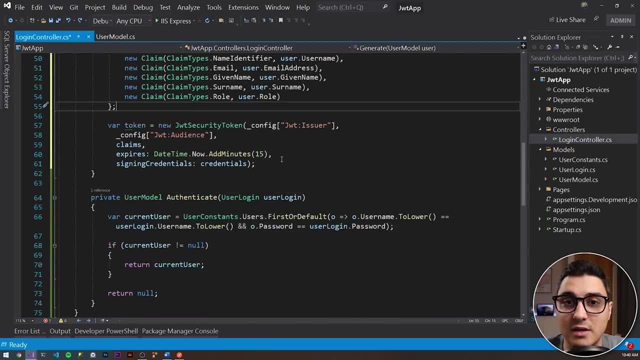 thing to do is to define the token object and what will it look like? and in this case, we're gonna be doing a new JWT security token and the first part is going to be the issuer, and it's important to pass the issuer and the audience, because this is what the API will validate once it read, once it. 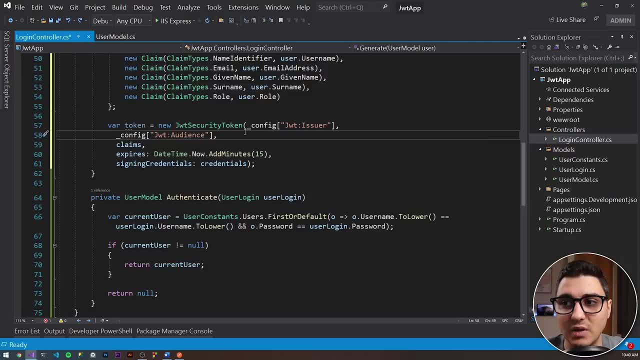 receives a request with a JWT token. so that's what we're going to do and we're going to define the JWT token. so it will check: has the issuer changed in the meantime from the one that you have defined in here, or has the? has the audience changed? 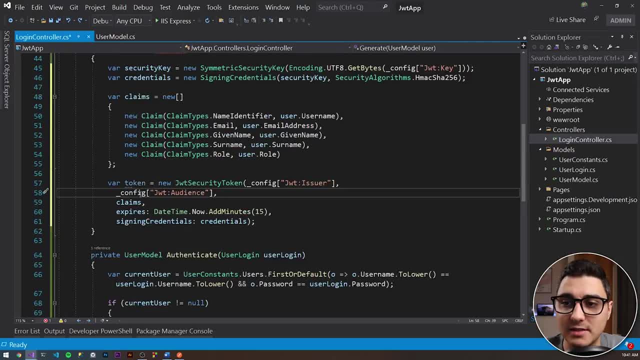 from the one that you've defined in the in the startup class. the next one is the list of claims- obviously we've already talked about them- and then when it expires, then it's recommended to do for a secure JWT token to not last more than 15 minutes, and then the signing credentials, which we have already. 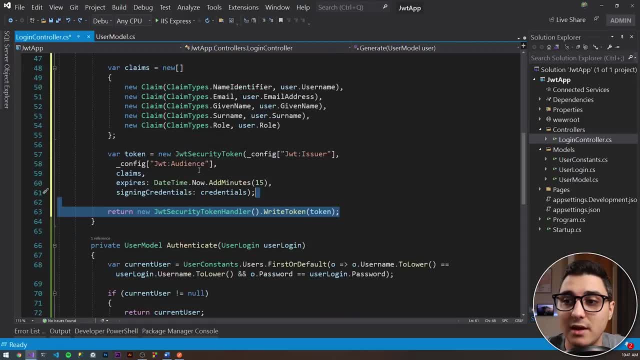 created right now. so that's what we're going to do, and then we're going to write here and that is it. so as soon as we have created this, you know, a JWT security token, then we call JWT security token handler and then we call the write token and we pass in the token object. so that's it. this should. 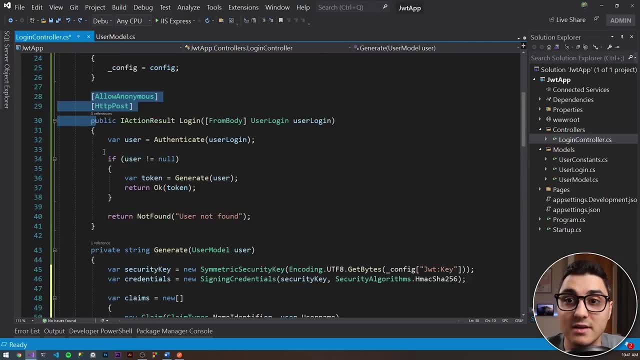 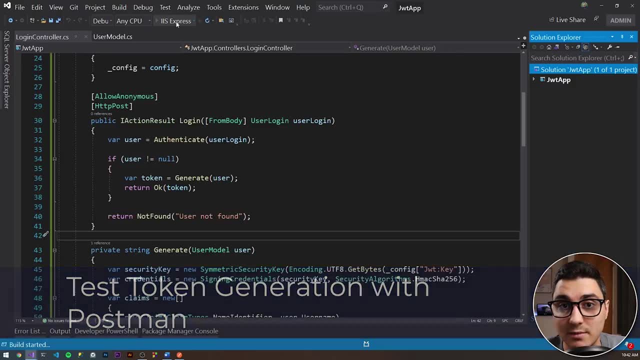 return a string now. so that is it with setting up our login controller, if you save, and let's quickly run the app and let's test what we've got so far to try to attempt to authenticate our users and let's generate a jot token so that we 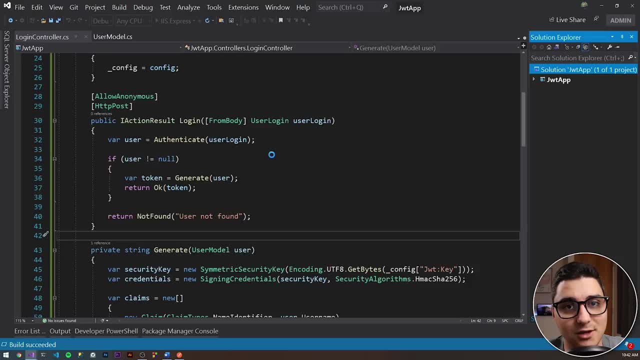 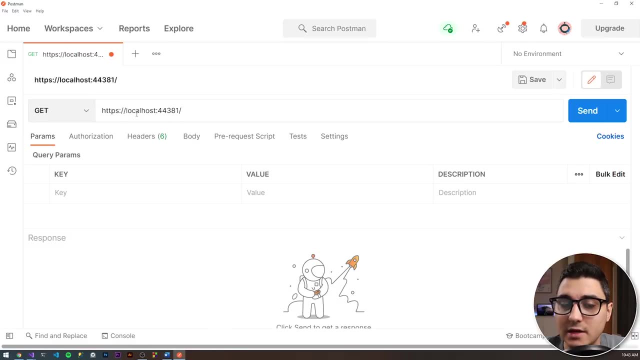 can get a hold of it and use it later on in this video. ok, so the app has started and if we copy the URL, that's attempt to login. so to login we do API, slash, API. so localhost, localhost, colon and then the port that you have in your, in your. 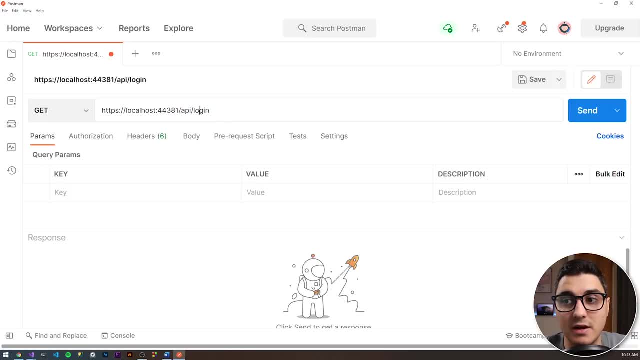 application URL and then slash API, slash login and then in here to be able to log with the username and password. let's go to the body tab, then let's go to raw and let's select json. so then in here let's log in with json admin and let's see if we can hit this login breakpoint. 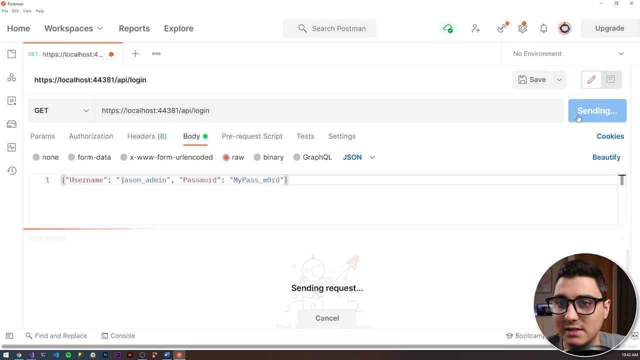 now. so let me put a breakpoint right here and let's click send. so this is a get method and it's gonna do a method not allowed. let's select the post method because that's what we defined inside the api and it looks like we've hit the api. so let's step into the authenticate method. 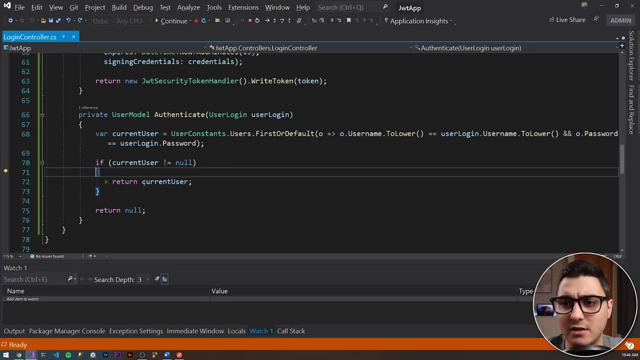 obviously compare the username and the password and the user is not going to be null. so just return the current user with all the details that we have defined in the user constants class. define that, so yeah, so get that user and then, if it's not null, obviously go in the generate. 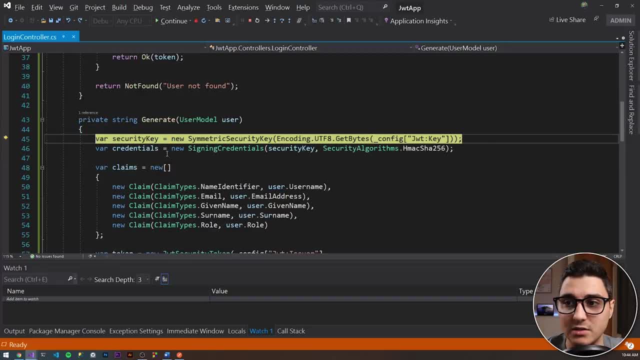 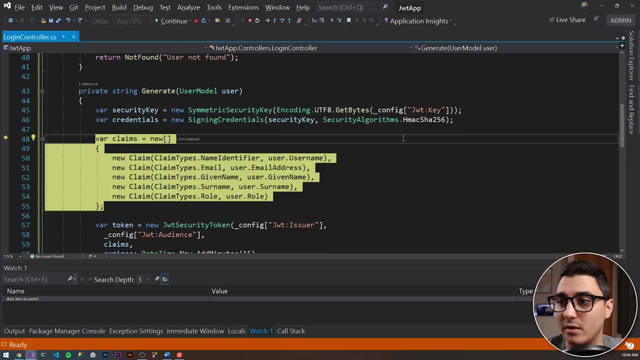 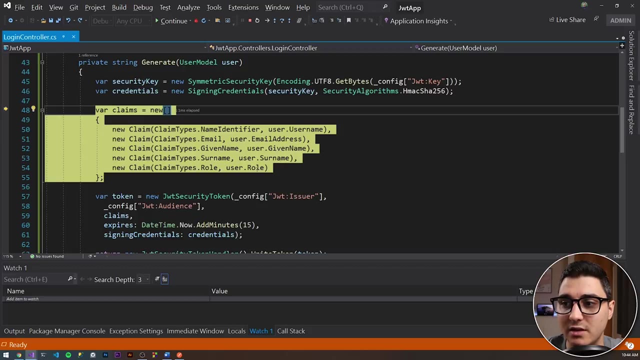 method and generate me a job token. so grab the security key- this is what the object looks like- and then define the credentials that we're gonna chug into the job token. define the, the claims. this is the username, the email address, given name, surname and the security role. so then define. 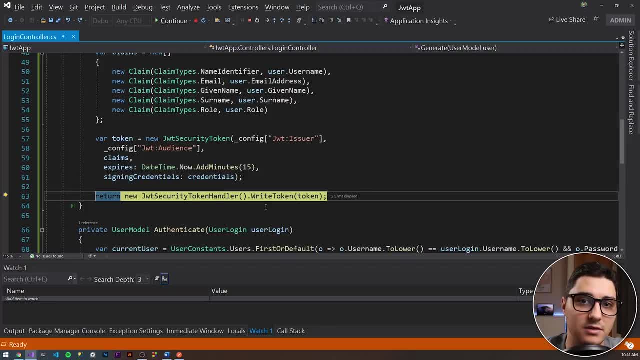 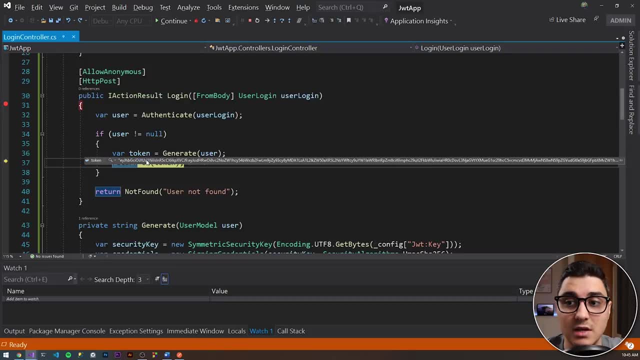 the jwt security token and then write it, so, in essence, generate it. so here we go. this is, this is the um, a string, the job token that we're gonna be using to be able to authenticate, to be able to let the api um authenticate and recognize the fact that we are authenticated and validate our um, our identity. okay, so if we 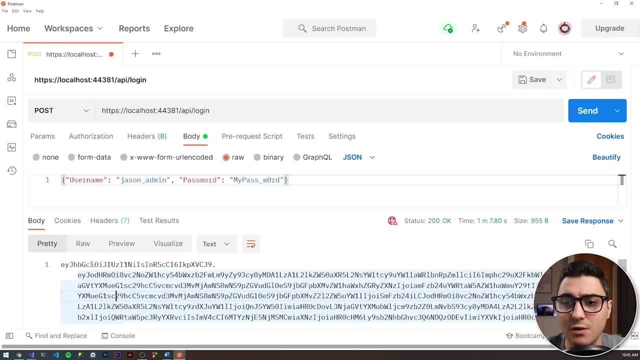 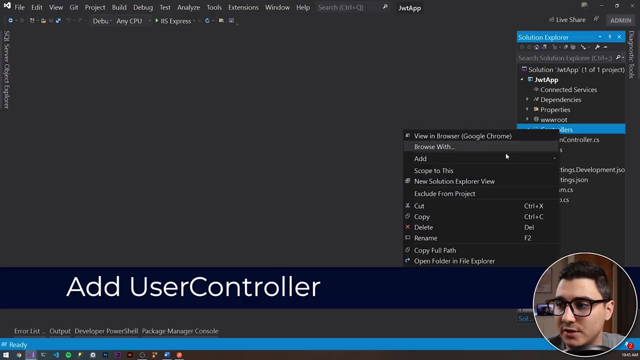 continue. if you can see in the in the body right here, we have got the dwt token uh generated for us. next, what we will do, we'll set up the user controller, okay, so back in the application. let's stop the app uh, close the login controller because we won't need it anymore for this tutorial. 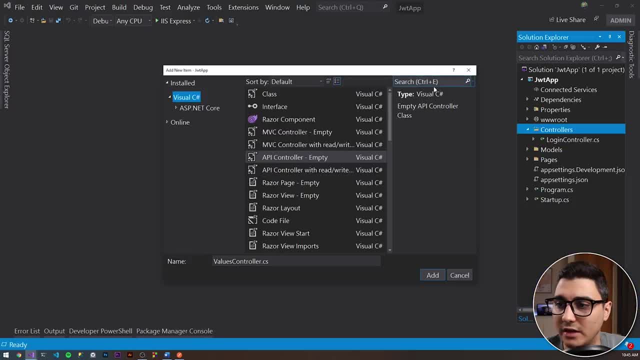 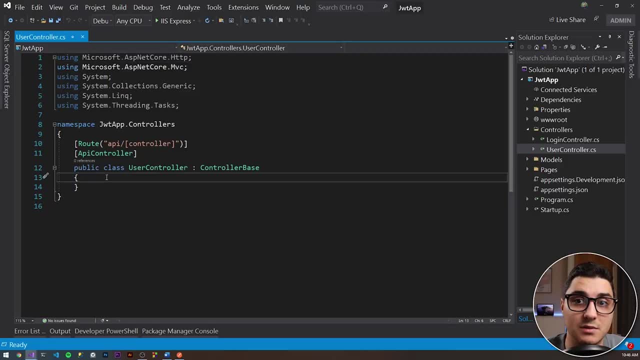 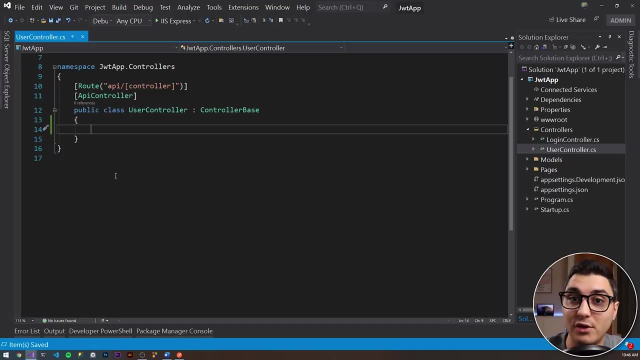 and then add, and then new item, and then again new api controller, and let's call this a user controller, and we're gonna, we're going to define a bunch of endpoints as part of this user controller, um, to be able to show whether or not we can hit those endpoints if we are authenticated and if we're not, what happens? so the first thing, 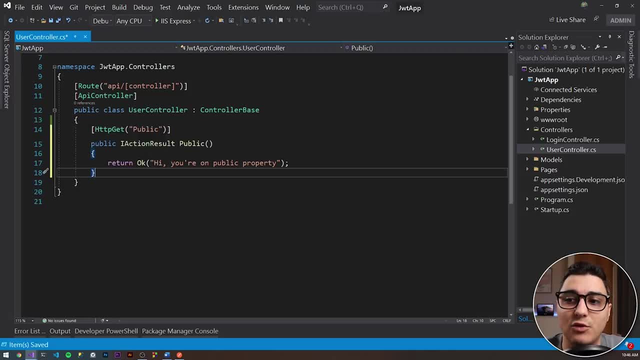 that i would like to do is let's add a public endpoint right here to say, hi, you're on public property and let's try to hit that checkpoint. what i would like to do here is switch to an orthography right here, are able to say: hi, you're on public property and let's try to hit that checkpoint. 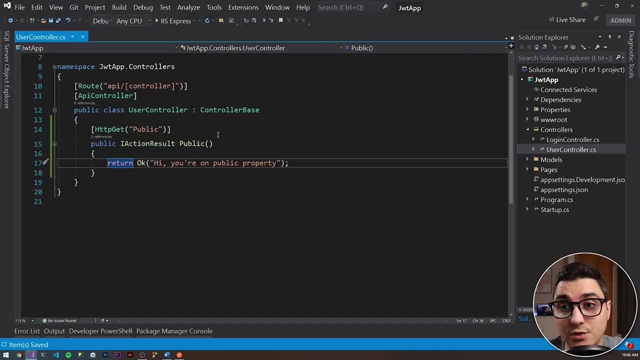 so i have his password. like i mentioned earlier, if we're authenticating, then um, and so that gives me to make to make sure that we are actually able to hit methods inside this endpoint to alleviate the confusion. so let's run the app and let's go back to postman. let's try to hit this endpoint, okay, so 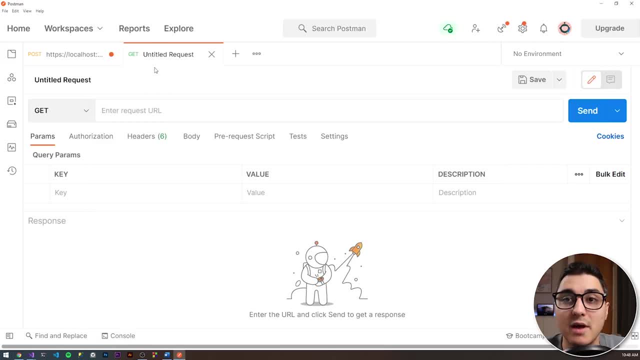 the app has not started and, um, if we copy the url, go back in postman and then open up a new tab and then let's paste that in there. so this is going to be api slash, user slash, public, and this is going to be a get method, so let's send it and let's see what we've got. hi, you're on public property. 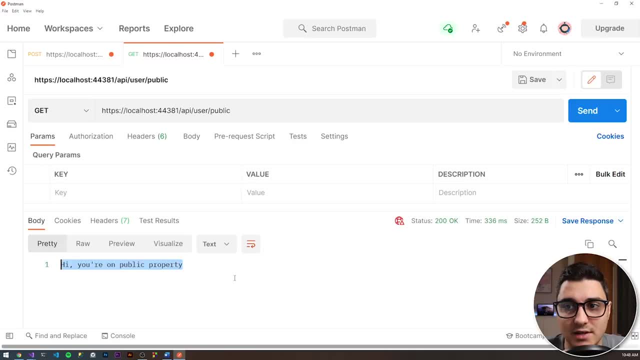 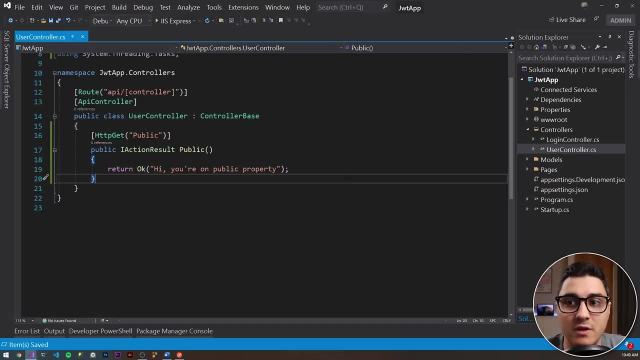 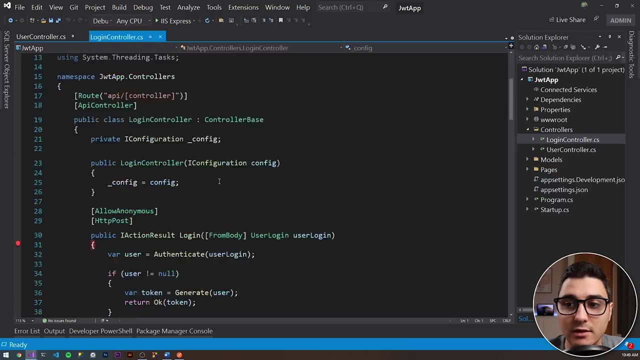 so we are now able to hit endpoints inside that uh controller. okay, so back in our application. uh, let's add a helper function that will allow us to grab the user details based on the jwt token uh passed in. so basically, when we were in the login controller, if you remember. 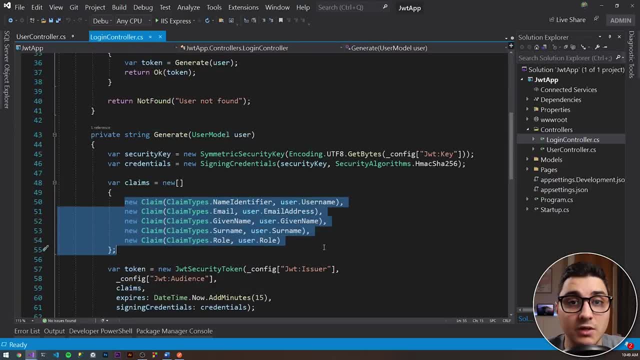 we have defined a bunch of claims. basically these claims hold useful information about the user without us having to go back to the database to to request details about the user. so every time you make a request, you send with the request that jwt token that holds all these useful details about the user that we can. 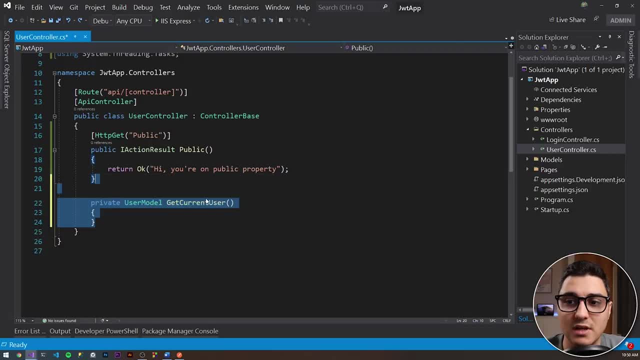 use inside our um example user controller. so the first thing, uh, let's define this as get current user and uh, we're gonna grab the identity from http context dot, user dot. identity as claims identity, because this is what it is, and if that is not null, then um. 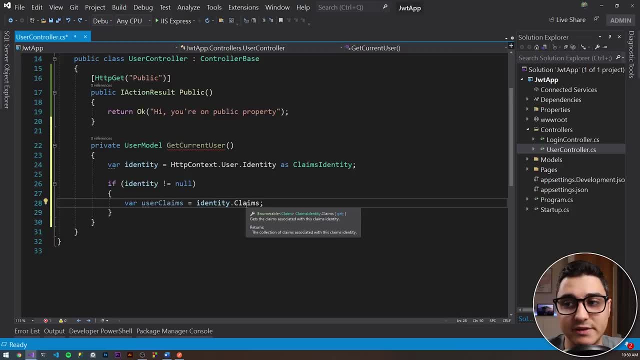 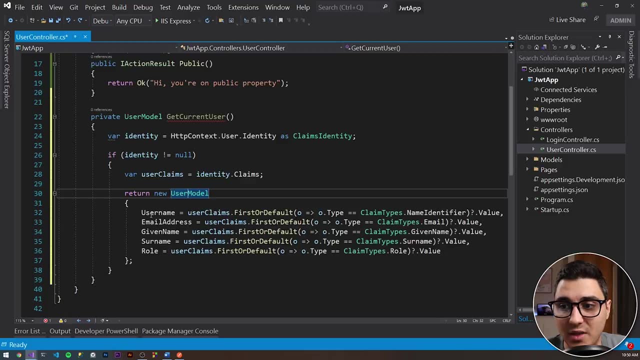 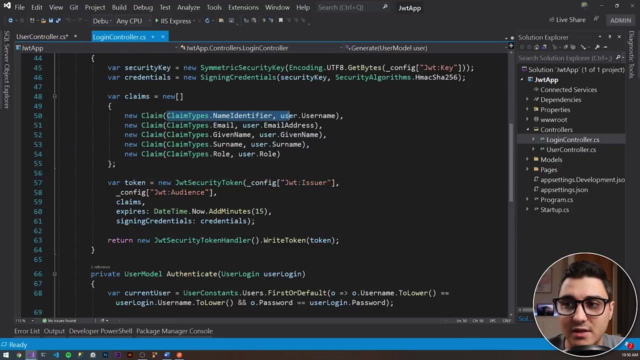 claims, array of claims, and this is basically just an innumerable of claims. and then let's create a new user model based on the claims that we have. so if we we are looking through the, the user claims, and we're grabbing based on type, so, if you remember, we have defined in the user controller certain types and 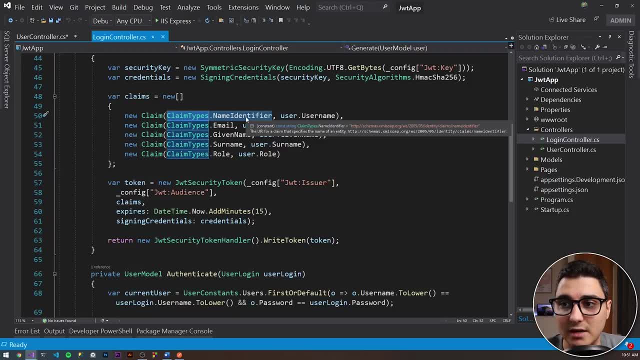 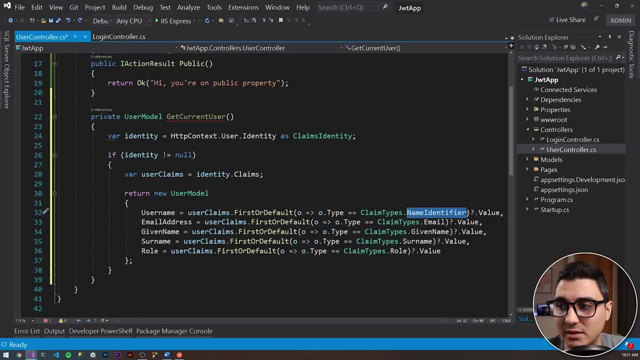 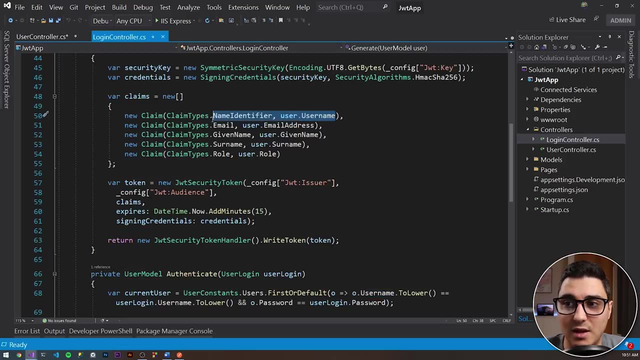 these are registered claim types and we are doing the same to be able to identify those types. so if the type is name identifier, then grab that, grab that value and put in the username property of this object. so, as you can see, we have stored the username in the name identifier and we're doing exactly the 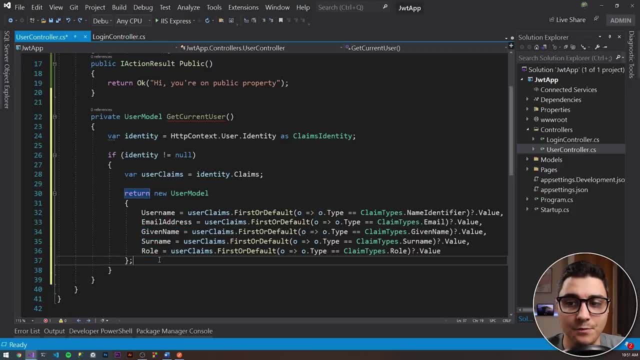 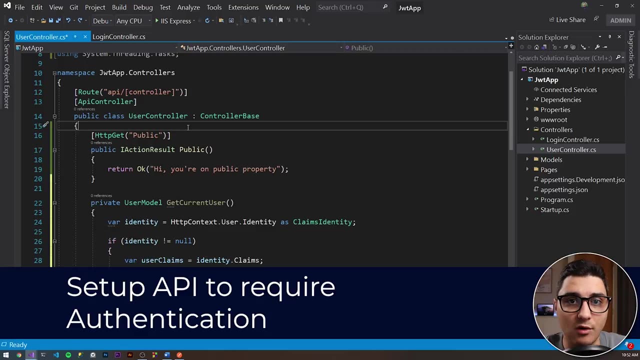 same thing with email address: given name, surname and the security role and then return null. basically, if if the identity is not found, then return null. so this is really useful because we're going to use this quite a bit in the following minutes. ok, following, let's define an endpoint. 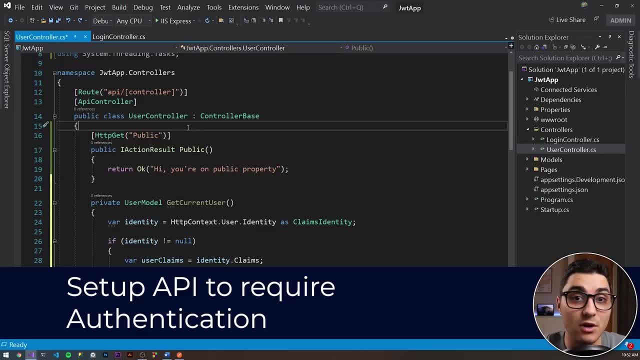 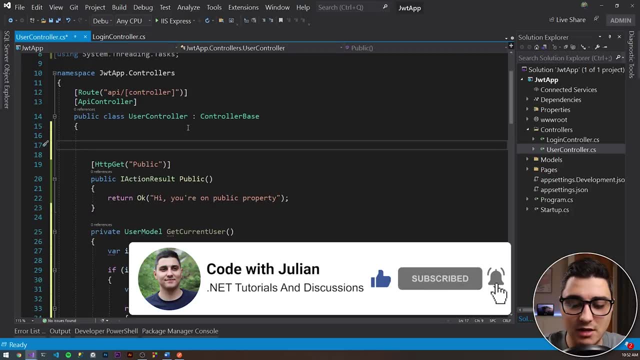 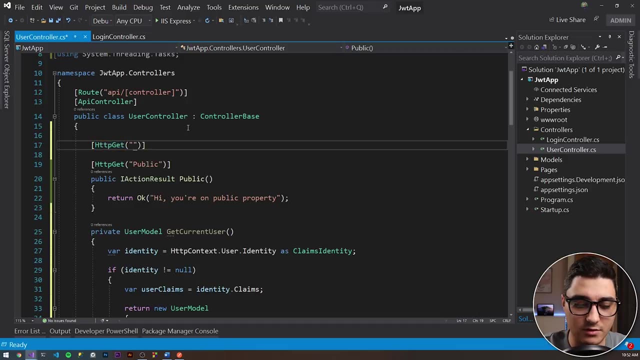 that will actually require us to be authenticated. so we're not going to be able to access that endpoint unless we are authenticated. and this is going to be again HTTP method, so HTTP get, and then the route to this will be: say: admins, yeah, because we're going to use 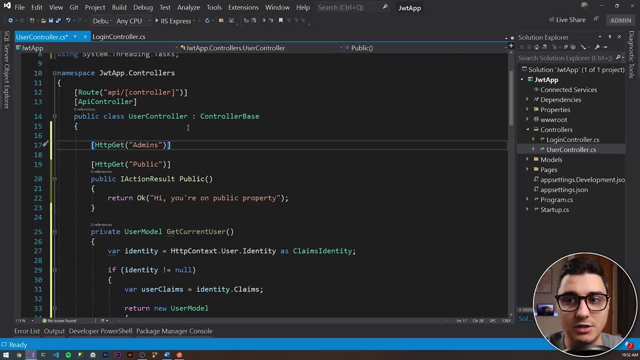 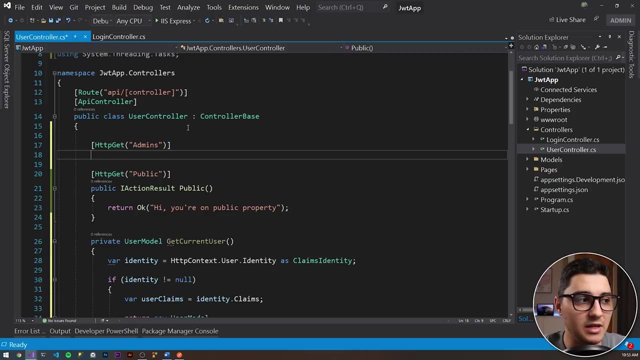 W исторico. yeah, because we're going to use W, going to actually um. after this. we are going to um add authorization. so only if you are an administrator you can access this endpoint, but for now you should only be authenticated, so you should only have a valid uh token. uh, okay, so this is a http guest get and then this is going to be a. 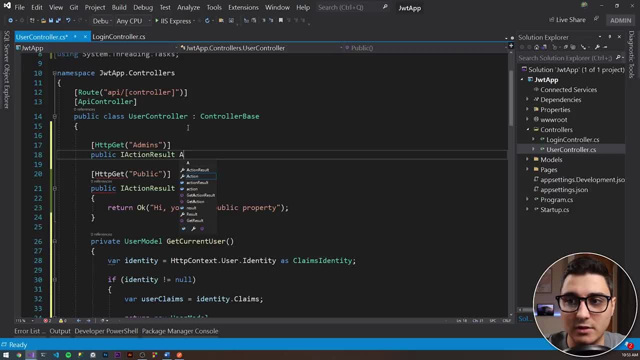 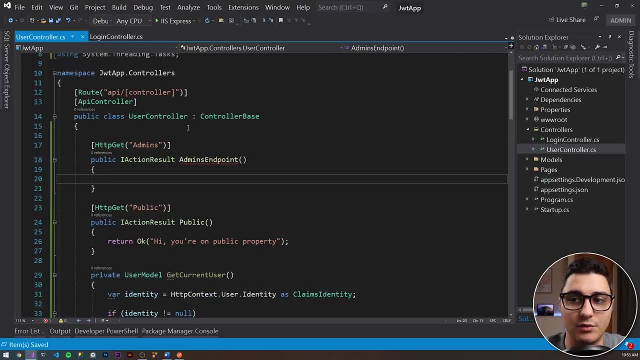 public eye action result: uh, and let's call this admins endpoint. it won't make a difference again, it won't make a difference. your security role at this point? um, so then in here, let's grab the current user. current user, that's going to be get current user. so this method right here and we. 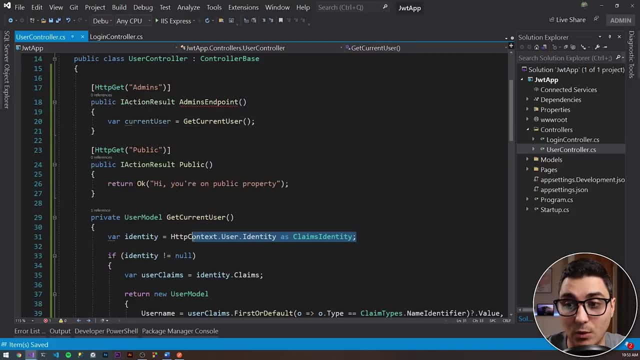 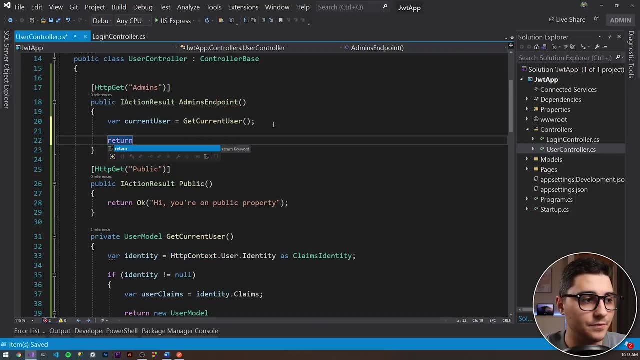 don't need to pass anything in, because this grabs the user claim. so all the details from the http context. so let's, let's just return in an okay message. if everything went okay, let's say hi, and then let's give the current user um given name and then let's say: 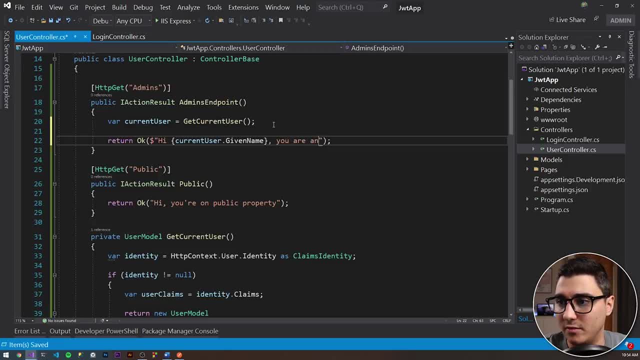 um, you are an and um or a um, and then let's put in the um security role right here. so, current user dot uh role, yeah, um. and then basically in here: uh, it will say something along the lines of: hi, jason, you are an and um or a um, and then let's save this, let's run the app and let's see, uh, what we've got. 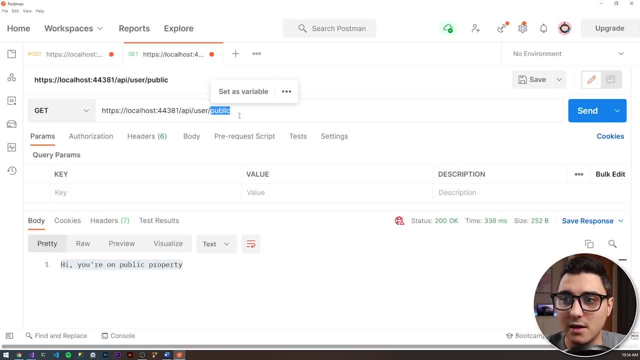 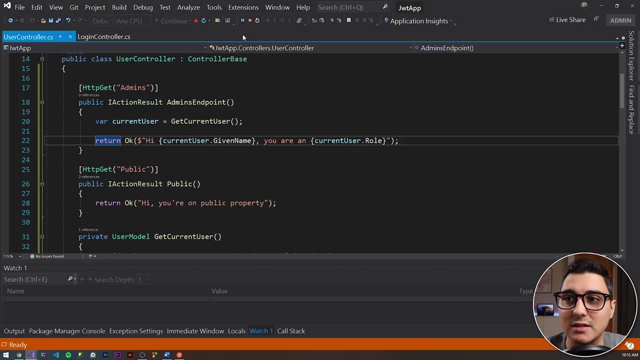 okay, so, uh, we're back in, postman, the app has started and uh, in here, let's um target the admins, uh, endpoint, and let's click send, and uh, what is going on? so, basically, we are not authenticated and we are able to access that endpoint. well, that's because we haven't added, uh, the authorize. 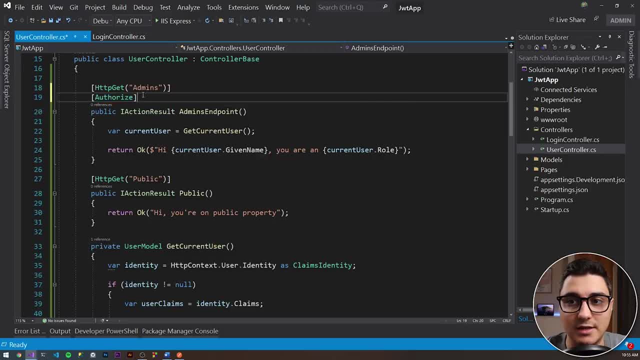 authorize um notation right here. so basically, we need to add this authorized in order for the api to validate the stock, and that's the whole deal. so, uh, at this point, if we have a valid jwt token generated and passed along with the request, then we will be able to access this endpoint. failing that, we won't be able to. so 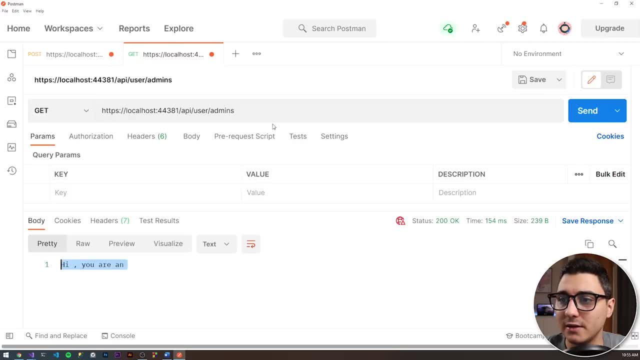 let's try that again. okay, so the app has started. and uh, let's try that again. so you'll see it returns a 401, unauthorized, and uh, to be able to access that endpoint, we're going to have to do a lot of things to do. to access that endpoint, we need to be authenticated, meaning that the jwt. 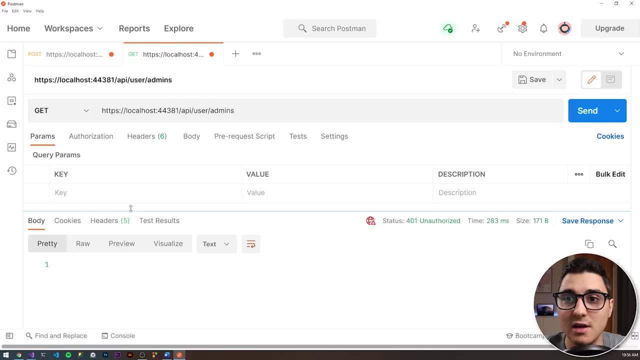 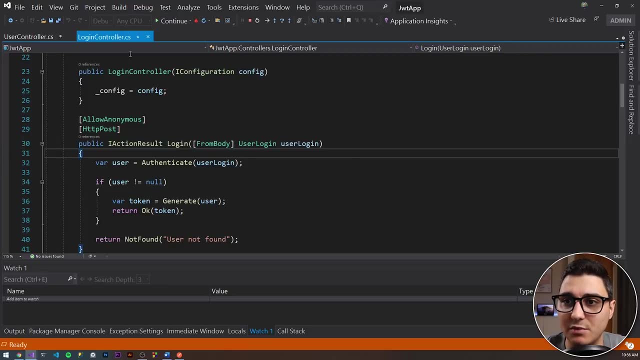 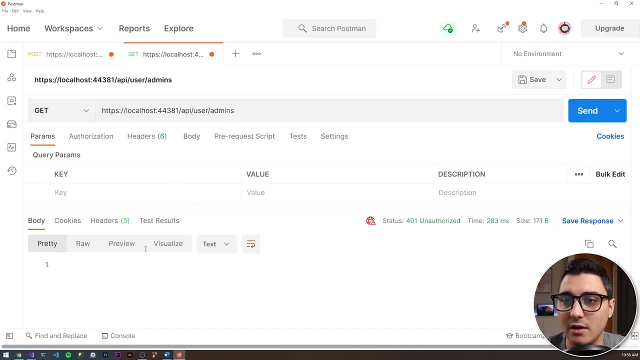 jwt token needs to be passed in along with the request. so if we uh go back in here, let's, uh, let's actually generate a brand new one. it's not been more than 15 minutes, but, hey, we want to make sure that that actually is a fresh, newly generated token with the json administrator. um, okay, so then. 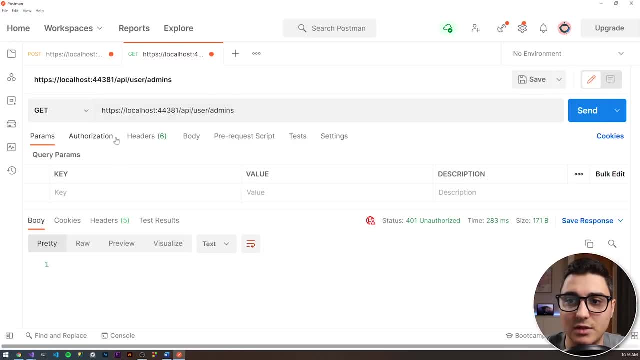 in here. we need to go to um instead of just sending this as it is. we need to go to authorization and type of authorization, choose bearer token- uh, and then paste this: uh- new security key- so yours is probably going to be empty like that- and then paste that um- a job token, not security key- job. 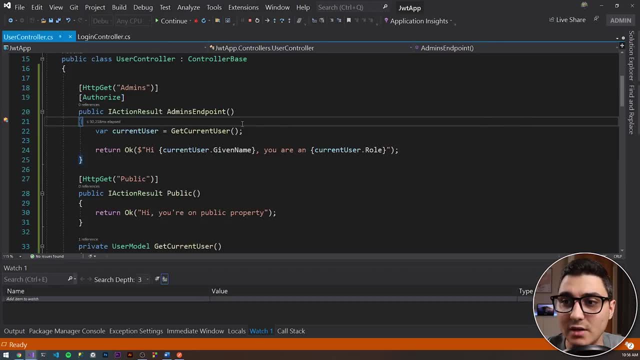 token. uh. so then let's try that again and, as you can see, um the api endpoint, the api has authorized this as we are successfully authenticated because we've passed in a valid fresh new token, generated so that the current user is jason admin with all the details, and we purposely don't didn't. 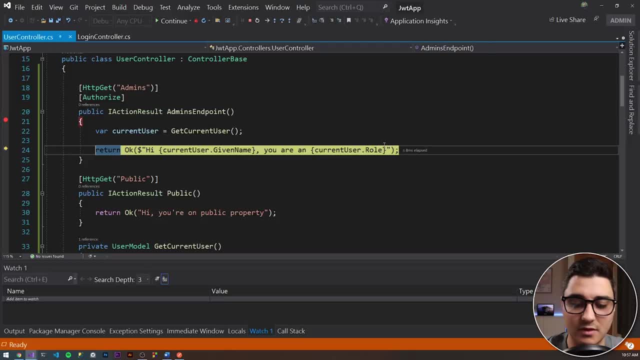 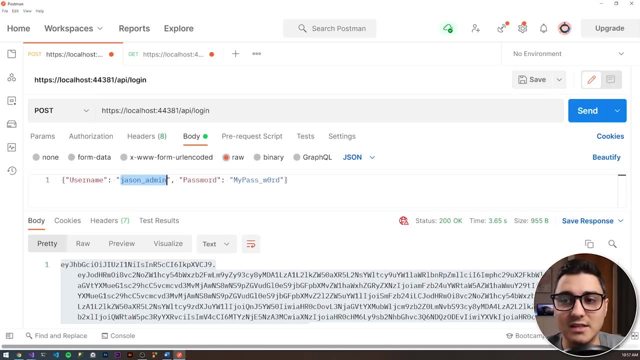 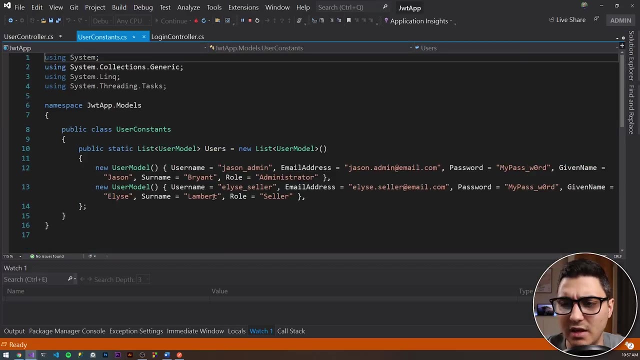 grab the password as well and, um, let's see what we've got. so, hi, jason, you are an administrator and obviously if we log in with elise, which will be inside user constants, so if we go and grab, they've got the same password. so, elise seller. 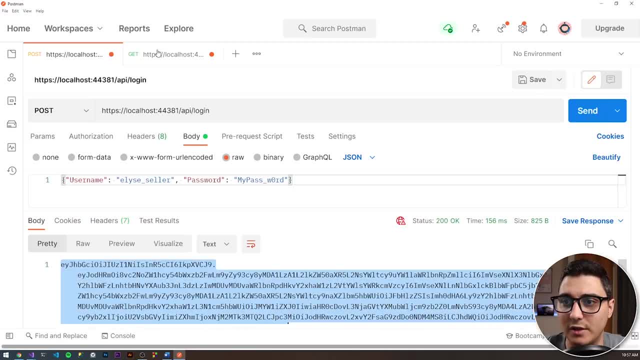 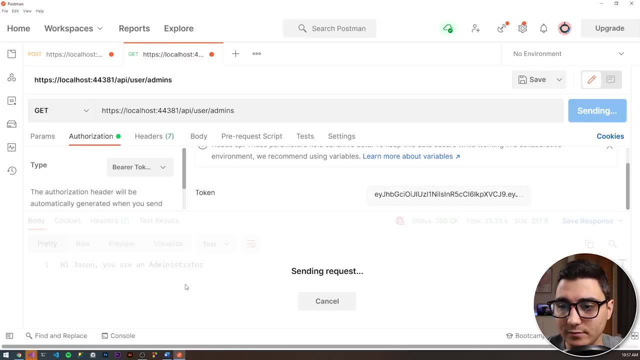 yeah, so if we log in and generate a jwt token with elise, uh, then replace this, replace jason's token with elise's token, then, uh, this breakpoint has already been. uh, hit, hi, elise, you are a seller, uh, and seller? well, that doesn't really matter at this point. um, because we haven't made the distinction between: 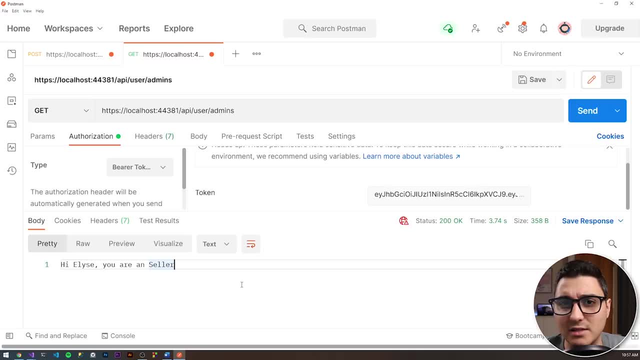 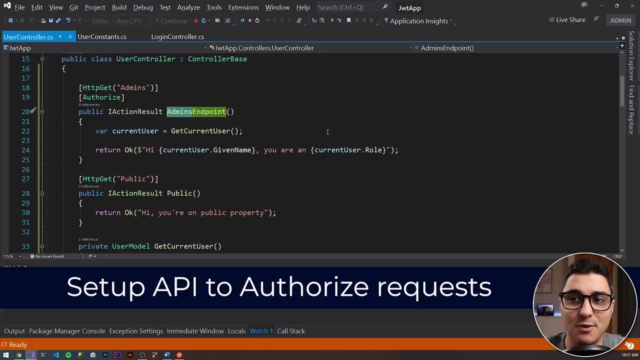 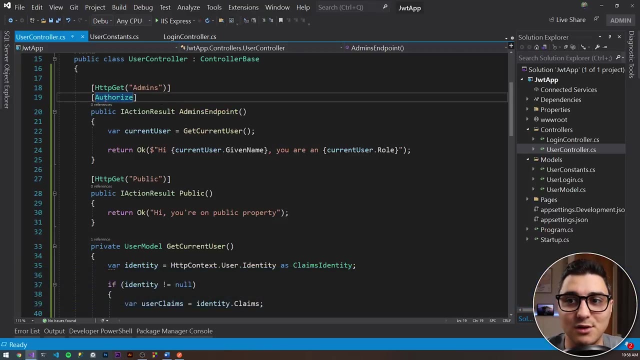 the two different security roles. uh, but how do you make a distinction? because this endpoint, surely, should only allow admins to be to be able to access it. well, basically, what you do is, in order to enforce um authorization between different security roles, what you do is open and close. 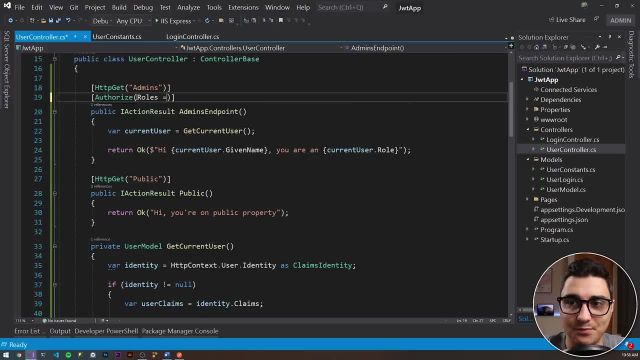 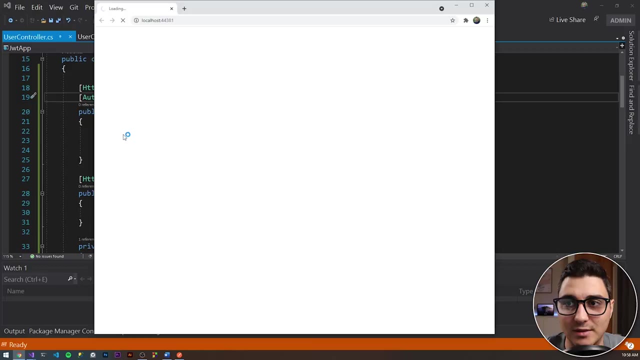 the parentheses and then you put you define the roles property right here. so this would be an administrator. so at this point, if we run the app, at this point, we shouldn't be able to access this endpoint with elise's generated token. so let's give that a try and let's see how it works okay. 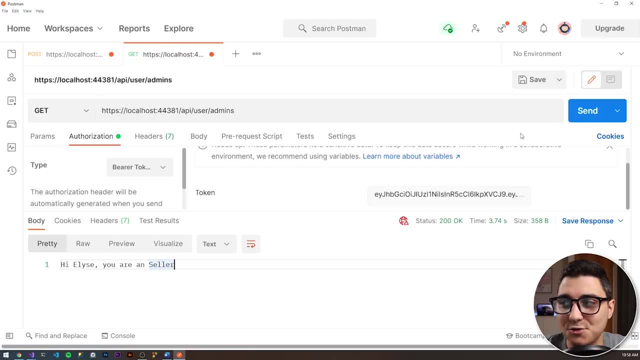 so the app has started. let's go back to postman and uh, let's try this again as it is with elise's uh token and uh, what you will see is not will not be a 401 um, it will be a 403, forbidden. so 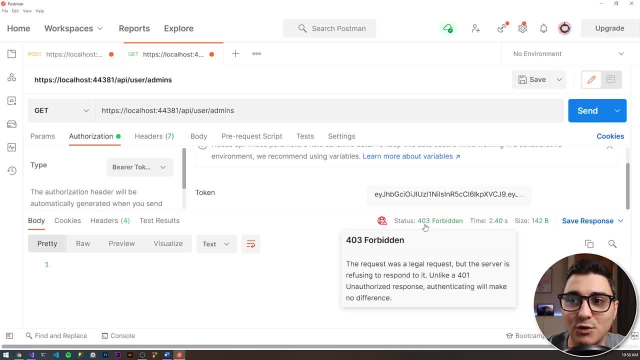 you are authenticated, but you are not who you, uh, who you claim to be, or better. yet this particular endpoint is not for you. you haven't got the right access or the right level of access, which we have defined right here, to be able to access that, and let's stop the application. 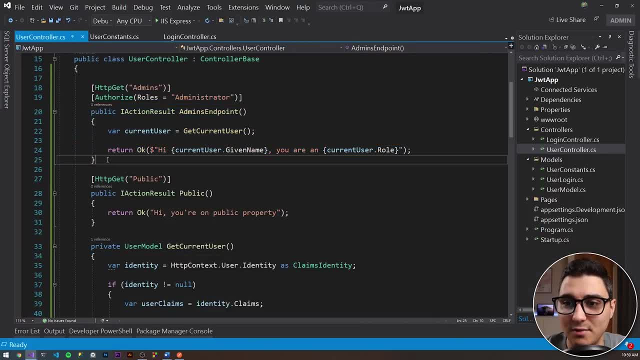 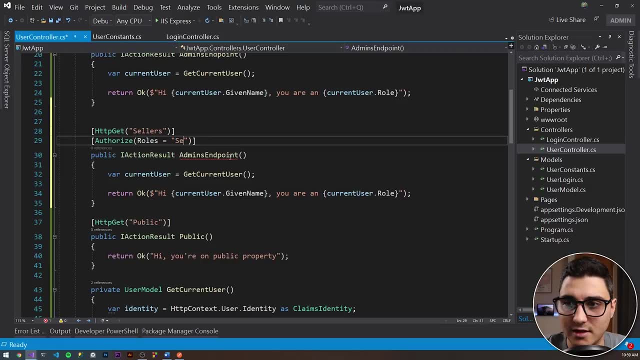 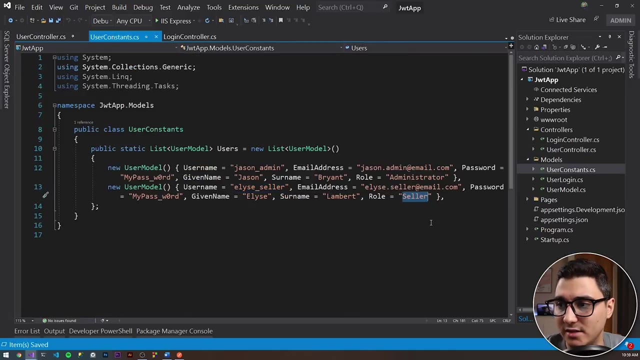 and let's create one for elise, uh, as well. so copy and paste this and this will be: uh, sellers, yeah, and then in here, let's define the role as the seller and, um, keep in mind this role. we have defined this role right here. uh, this is the elise's role, this is the seller and this is the. 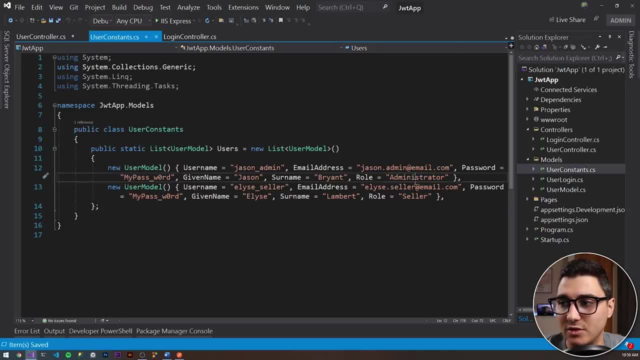 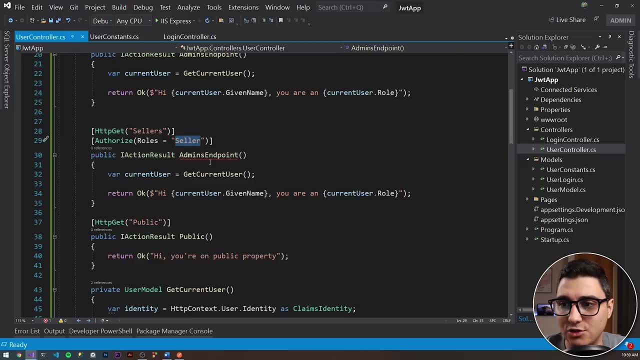 administrator, the jason's uh. security role. so basically, we have said that the role should be of administrator right here, and then, for at least uh, that it should be a seller. make sure that the names match: uh, right here. so let's call this seller, uh. seller's endpoint uh. so then here let's. 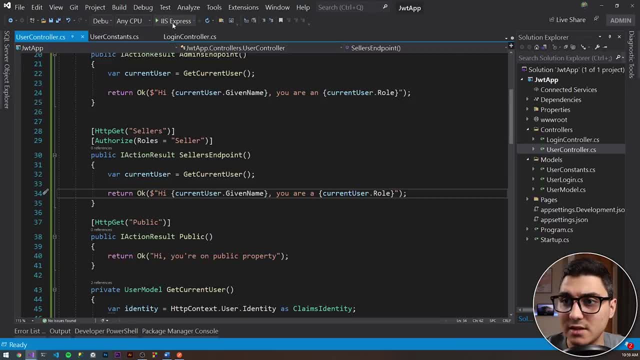 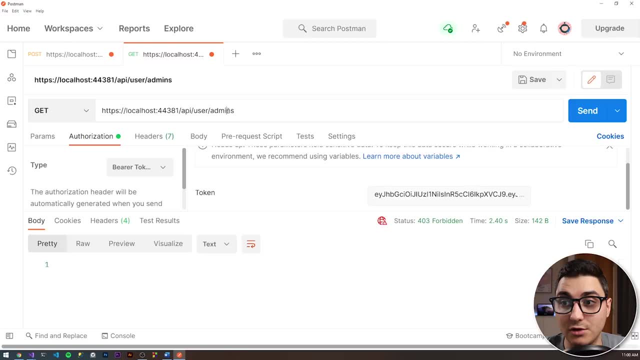 change this? um, okay, let's give this another run, let's see how it works. okay, this is right now, and uh, let's uh try. um. so again, the admins were not there, not going to be able to access the admins, so, um, nothing changed in that endpoint. however, if we say: 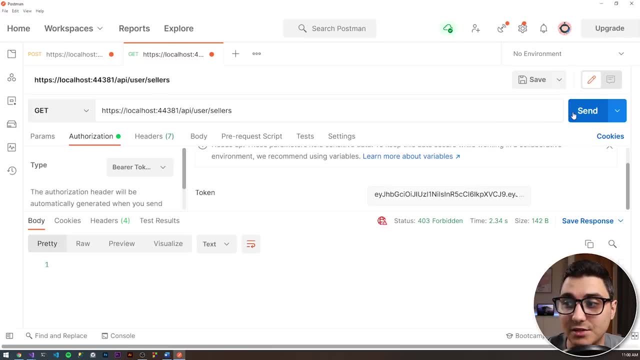 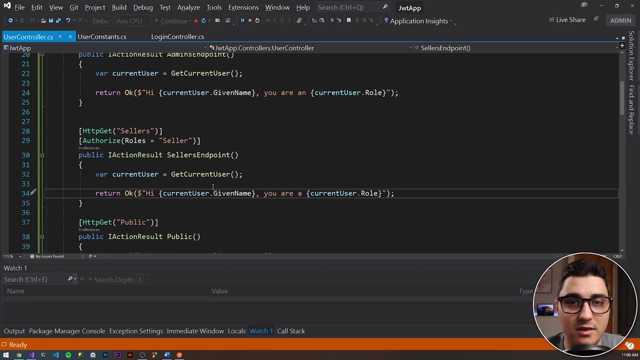 here sellers, so go ahead and access the sellers endpoint. uh, let's take a look at the response. so, hi, elise, you are a seller, so 200. okay, so it's been. we have been able to authenticate successfully and we have been authorized uh. so, in here, if we uh log in with uh, if we log back in with jason's.